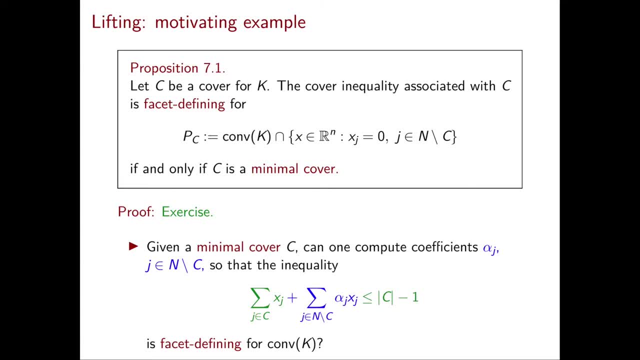 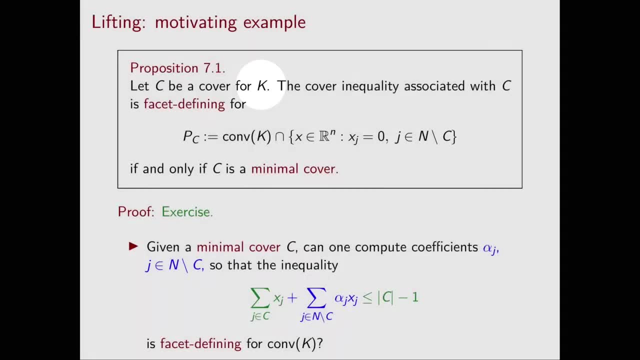 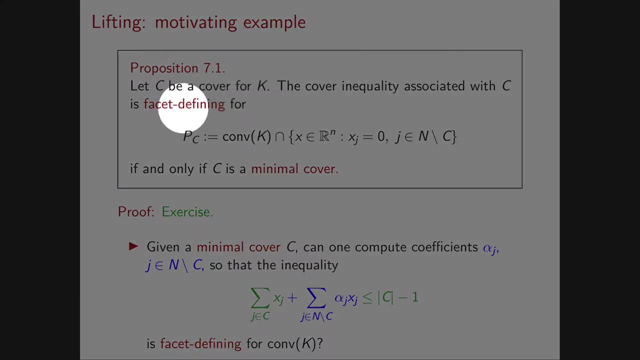 that among cover inequalities, the minimal cover inequalities are the strongest one. So let's read through this proposition: Let capital C be a cover for our knapsack set K. Then the cover inequality associated with capital C is a facet defining for this set Pc if, and only if, C is a minimal cover. 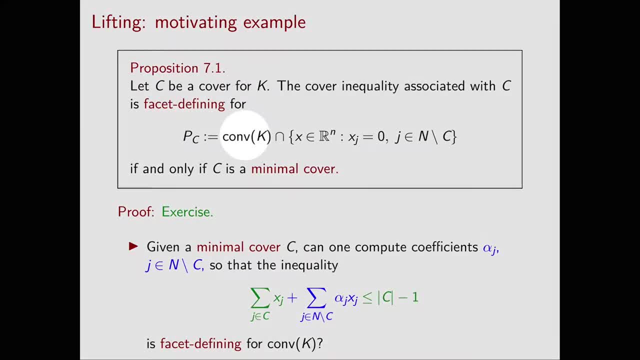 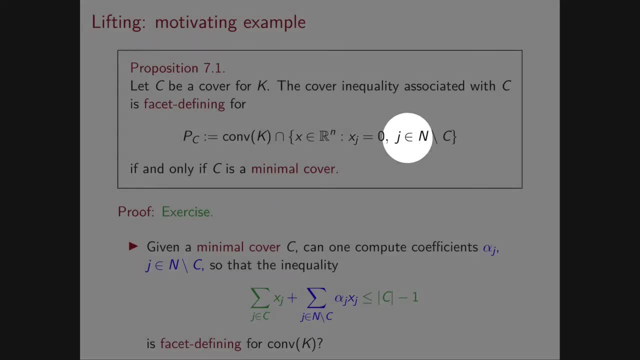 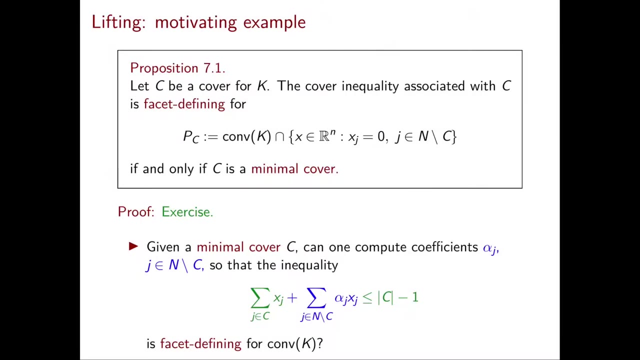 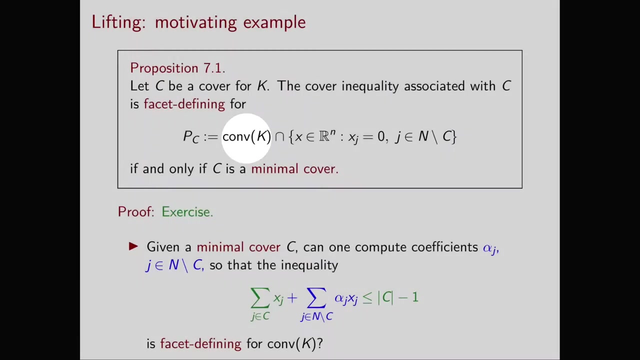 So what is this set Pc? It is the convex hull of K intersected with xj, equal to zero for every j, not in the cover. At this point, this set Pc seems a little bit technical. so this is a very interesting proposition. However, what about facet defining inequalities for conv K instead? And this is: 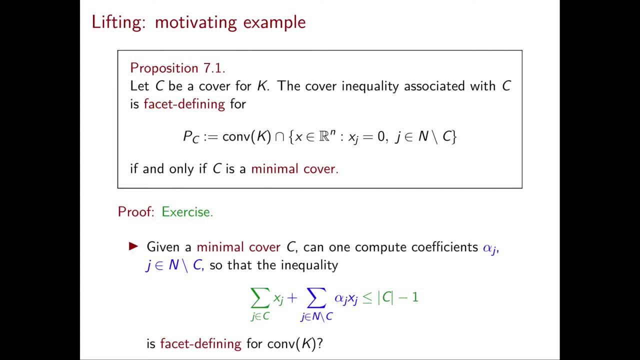 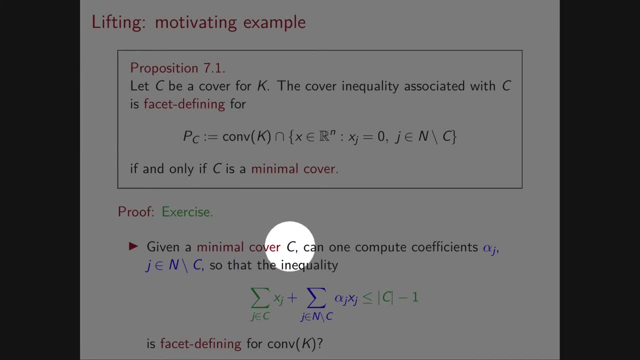 exactly the question that brings us, in a sense, in the direction of lifting. So let's pick a minimal cover C and the question is: can we compute coefficients alpha j for all the variables j which are not in the cover, so that the inequality obtained from the original minimal cover inequality? 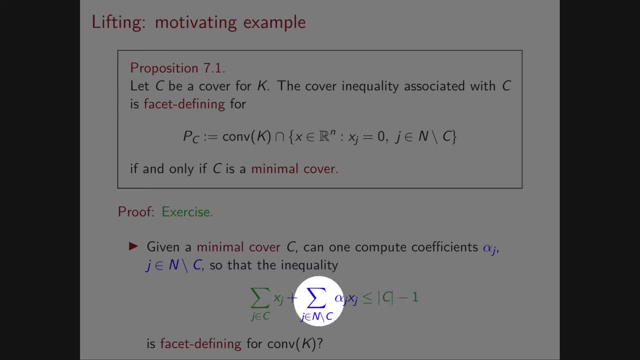 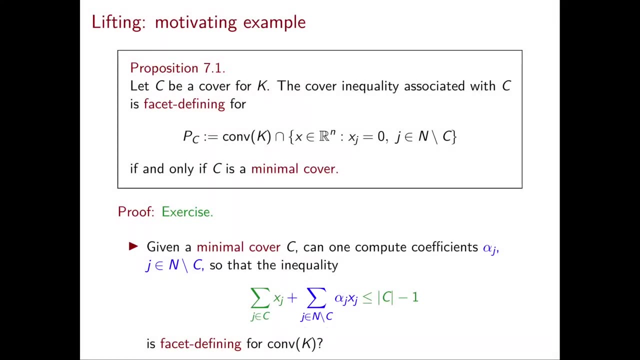 which is the one in green here. by adding the sum of the alpha j, x, j for all, the j in n minus c on the left hand becomes facet defining for the convex hull of K. We will see that the answer to this question is yes, but in order to get there, I want to do things more generally and not just for. 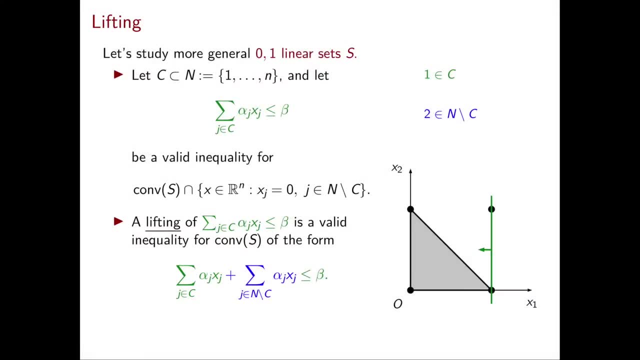 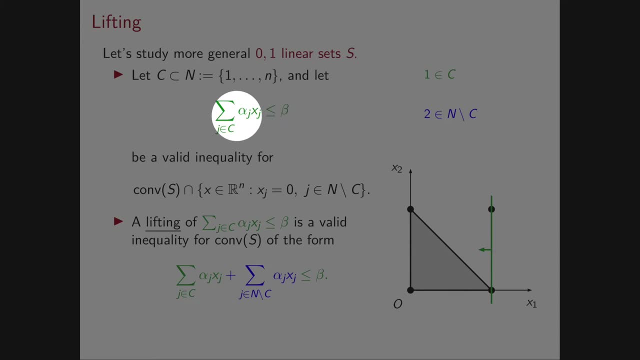 the convex hull of S. So let's look at the more general zero, one linear set that we denote by capital S. Then pick a valid inequality where the only variables that appear correspond to a subset- capital C, of all the variables, n, And let's assume that this inequality 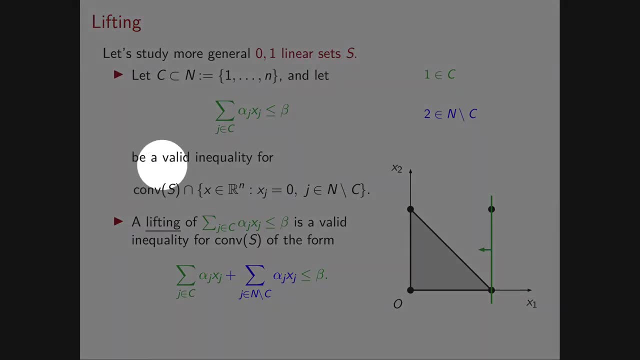 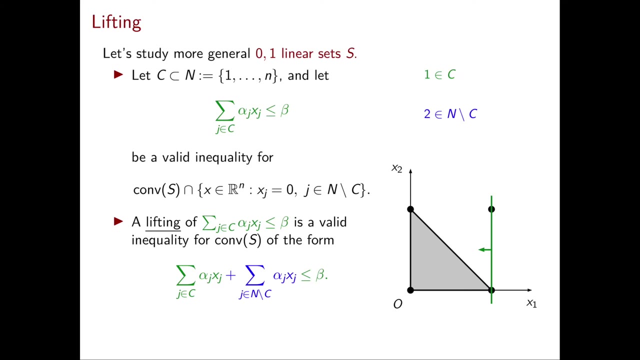 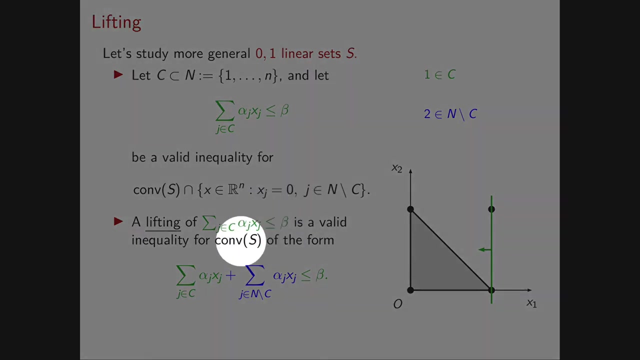 is valid for the convex hull of S, intersected xj equal to zero for every j that is not in C. Then we define a lifting of this green inequality and it's defined as a valid inequality for the convex hull of S of the form that we have here. So essentially it is exactly the green inequality. 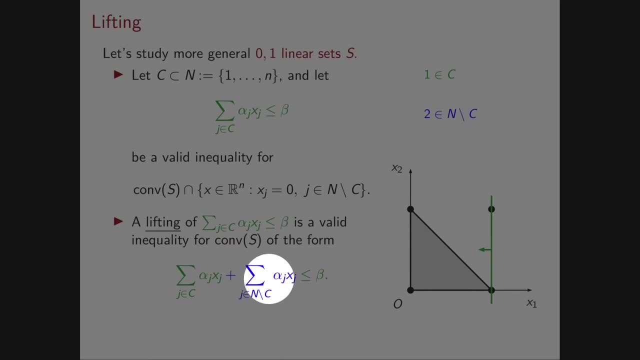 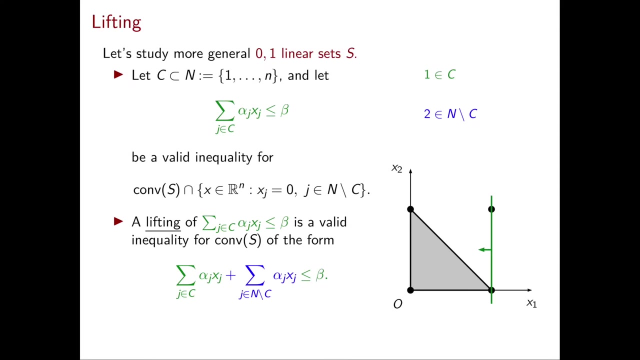 but where on the left hand, we are adding the sum of the alpha j, xj for every j, not in C. So let's see a couple of pictures that hopefully will clarify a little bit this concept. So here we just have a two-dimensional graph. 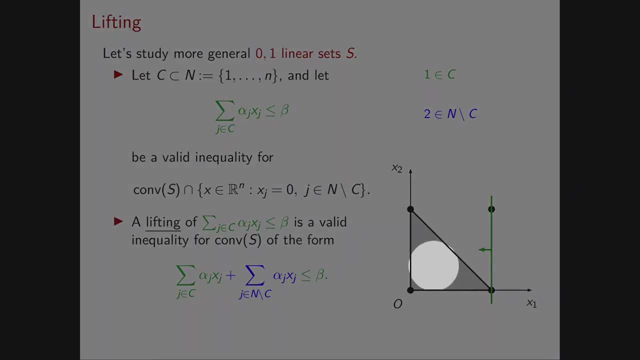 For example, this triangle is our set convex and in green we have our original inequality. Now we have that the index 1 is in capital C. In fact, this inequality is x1 less than or equal to 1.. So the only variable that appears is exactly the variable 1, which is in capital C. 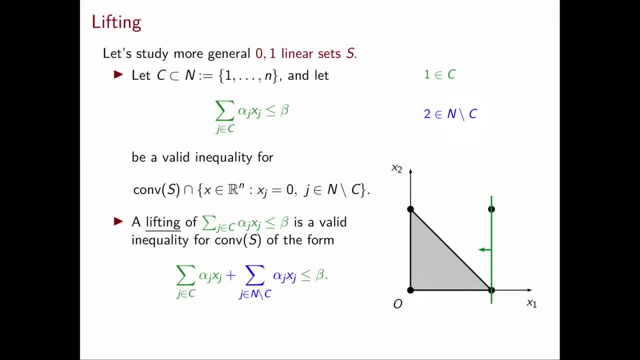 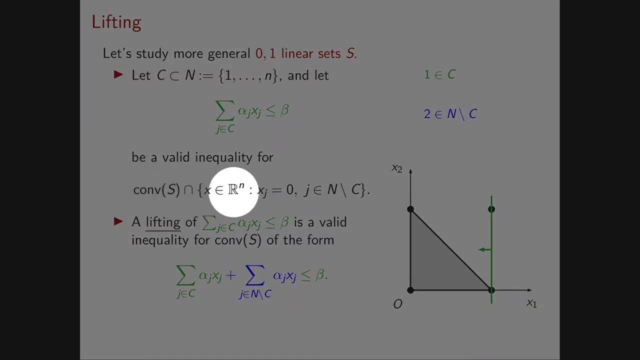 Therefore the index 2 instead is in n minus C. Furthermore, this green inequality is satisfied as our assumption because it is valid for convex intersected x2 equal to zero, And in fact this inequality is valid for the segment here between the origin and the point. So at this point, 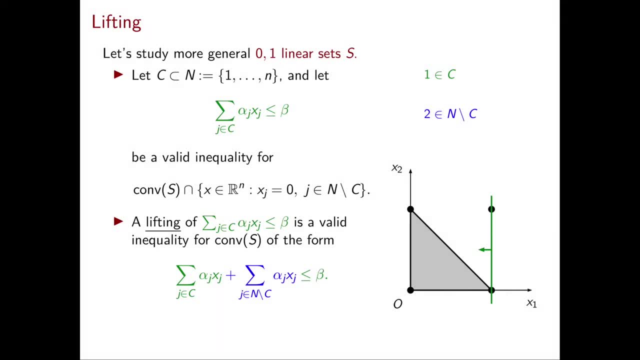 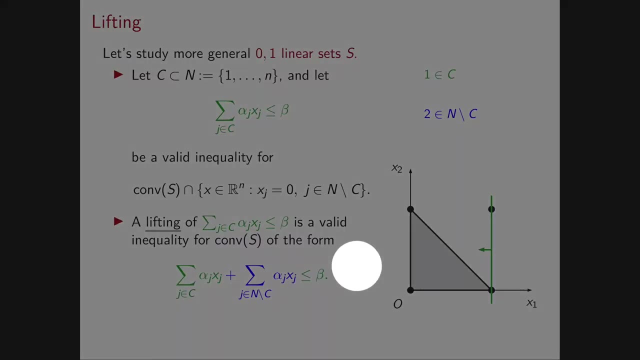 let's see some liftings of this inequality. One lifting that we can obtain is simply obtained by selecting alpha2 equal to zero. In such a way, the new inequality is exactly equal to the old one, So we obtain exactly the same inequality. So it is of this form. Furthermore, it's valid for convex, So it's. 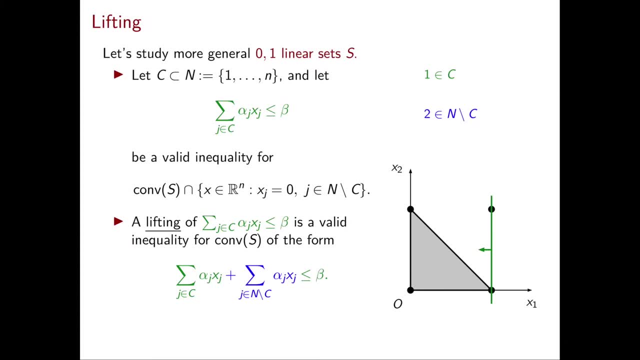 valid for the old triangle. So it's a lifting of the original inequality. Let's see another example, maybe a little bit less trivial. What about this blue inequality? In this case, the coefficient alpha 2 is definitely non-zero, And if the original inequality is x1, less than or equal to 1, this will. 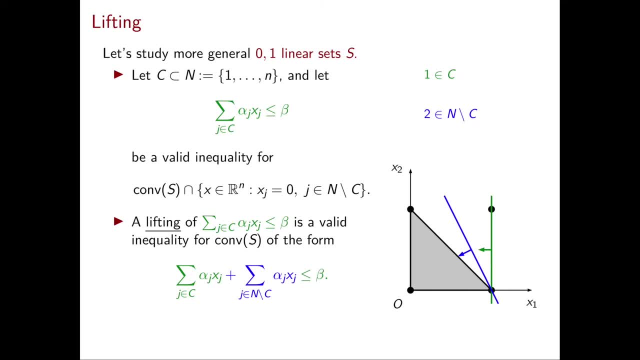 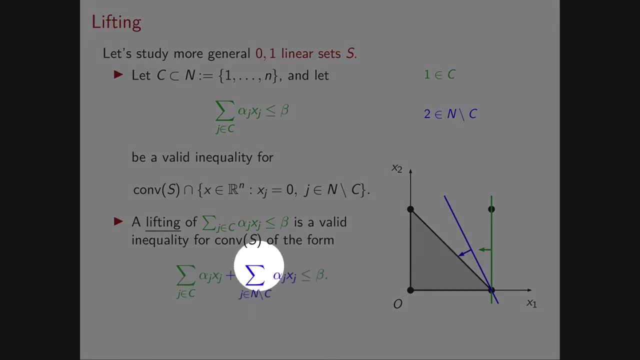 be x1 plus one half x2 less than or equal to zero. So the original inequality is x1 less than or equal to one. Also, this is a lifting of the original inequality. In fact, it's definitely of this form and it's still valid for the triangle. One important thing to notice is that the intersection 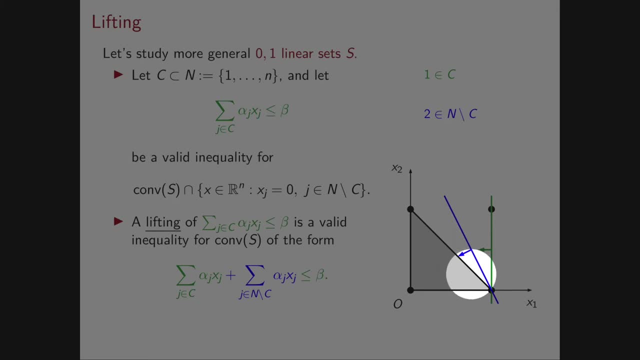 of this lifting. this blue lifting with the hyperplane x2 equal to zero coincides with the original inequality. And that's obvious because if you set to zero all the blue variables, you obtain exactly the old inequalities. So all the liftings must. 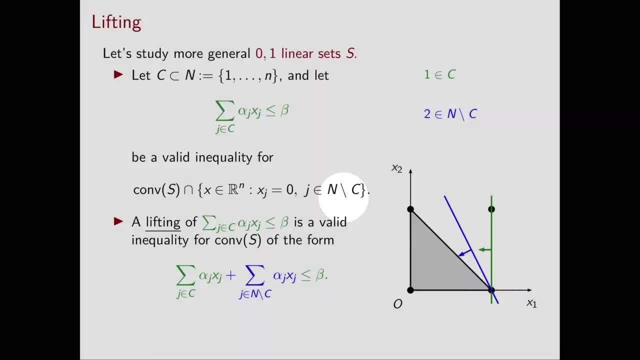 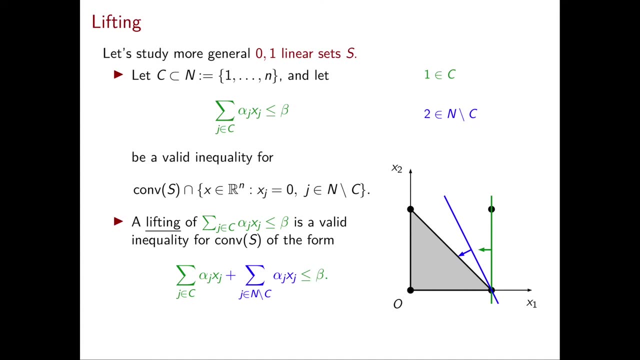 coincide on the hyperplane where we started from, And this makes us immediately understand that in order to obtain the strongest lifting of our original green inequality, we need to essentially maximize alpha 2 in this case. So this is the strongest lifting that you can obtain. This is the 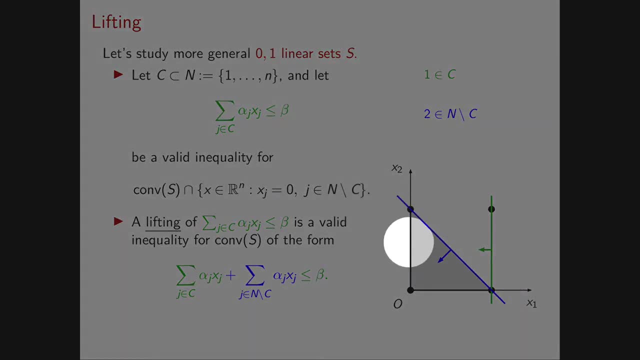 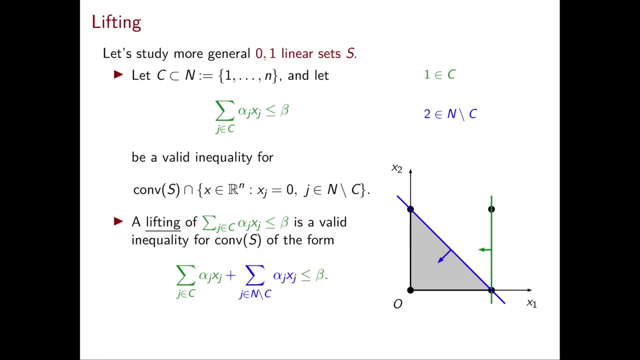 inequality: x1 plus x2 less than or equal to 1.. And it is a lifting of x1 less than or equal to 1 because it's of this form And it's still valid for the triangle. Let's now look at an example that is a little bit different. 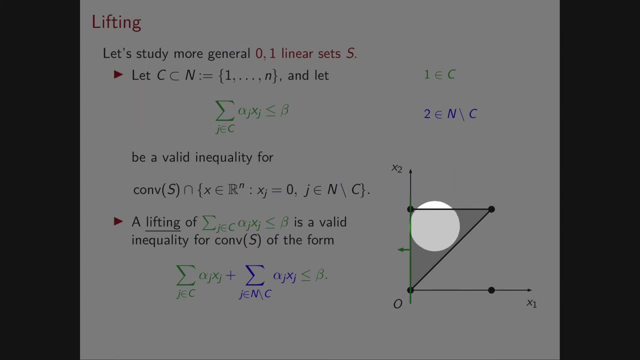 So everything I'm changing is that the triangle is now the convex hull of the origin, the point 1,1 and the point 0,1.. At this point we still keep 1 in c and 2 in n minus c, Therefore the green. 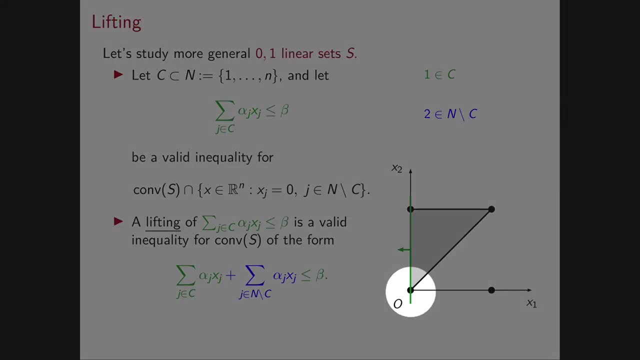 inequality could be, for example, x1, less than or equal to zero. In fact, it is valid for the triangle intersected x2 equal to zero. So the green inequality could be x1, less than or equal to zero. In fact, it is valid for the triangle intersected x2 equal to zero. 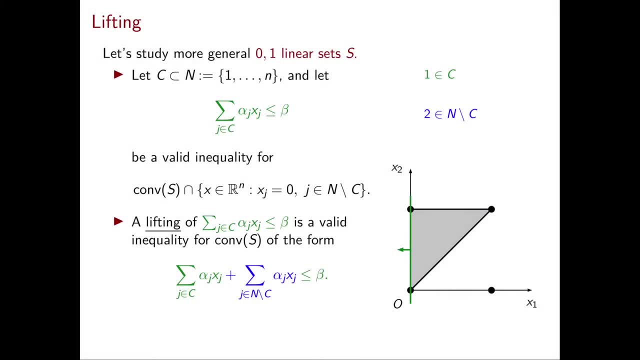 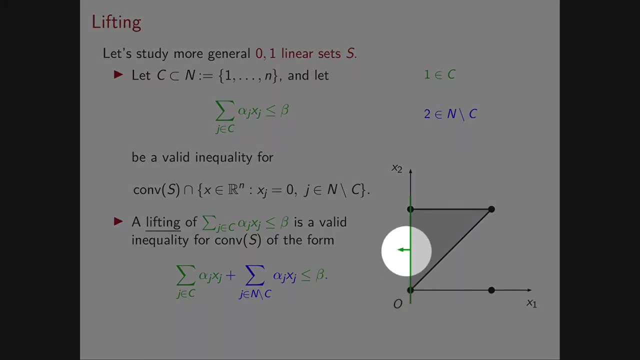 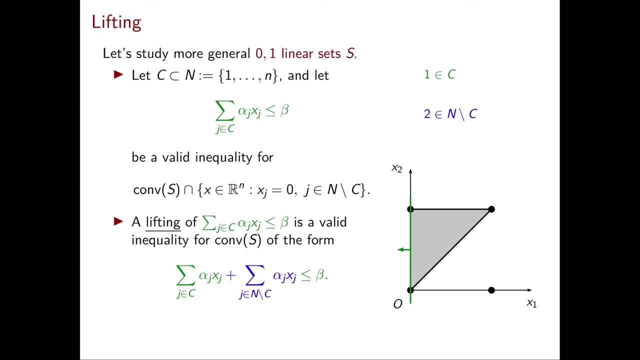 Which is just this point. So this is a bit less intuitive than before, but it's but highlights the fact that the inequality we start from is not necessarily valid for converse, but is just valid for a face of converse. In fact, in this case, the lifting obtained with alpha 2 equal to zero. 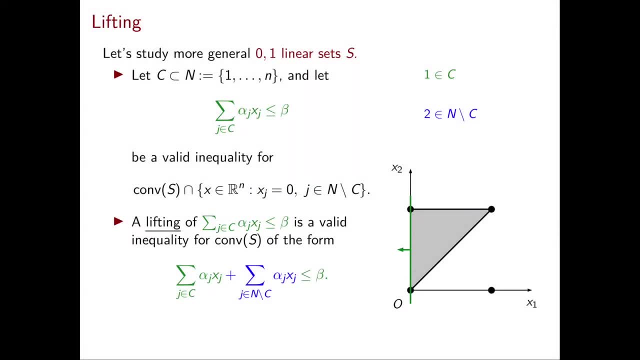 is again the same inequality and is not a lifting of the original green inequality. That's because it's not valid for the triangle. However, this inequality here in blue is instead a lifting of the original green inequality, because it's valid for the triangle and you can check it is of this form And also here in order to obtain. 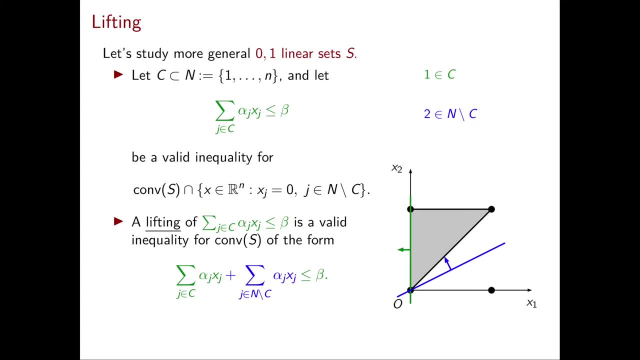 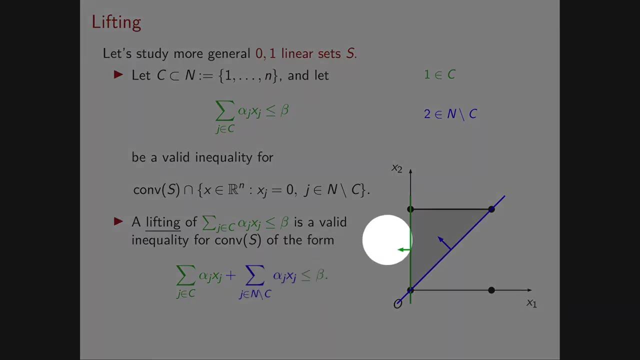 the best possible inequality, we need to maximize the coefficient alpha 2, and if we do so, we obtain this blue inequality here. We can already understand from these pictures an assumption that will be fundamental in our subsequent lifting theorem. In fact, in order to obtain a lifting, even in this picture, we need to 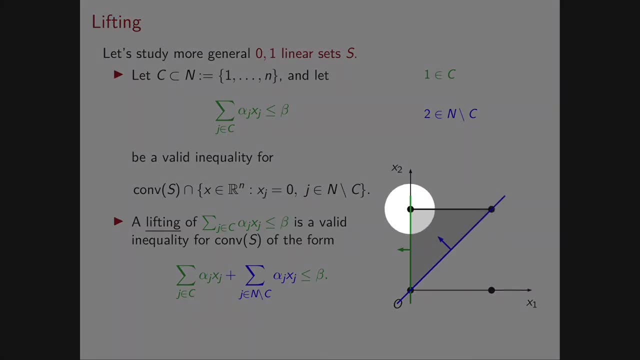 have at least one point in s intersected x2 equal to 1.. Because think about it, if we didn't have any- let's say in this case our polytope would have been only the origin- then, by maximizing alpha j, we can tilt this inequality all the way until it's exactly x2 less than or equal to zero. essentially, 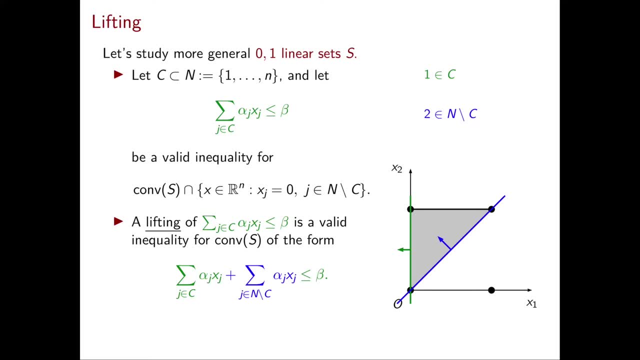 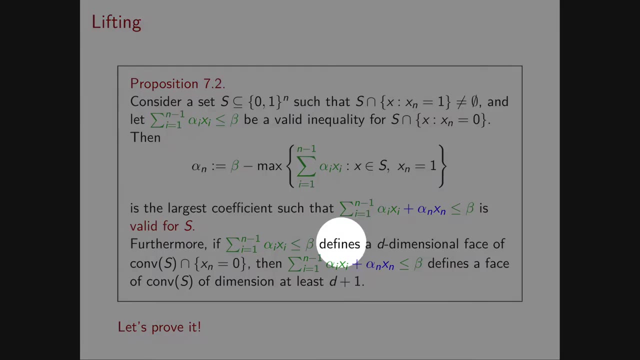 And at this point this is no longer a lifting of the original inequality. So essentially it makes no sense to lift in such a case. So now let's state and prove our main lifting result. So we have a set s in 0, 1 to the n. that satisfies this technical assumption that we just talked about. So 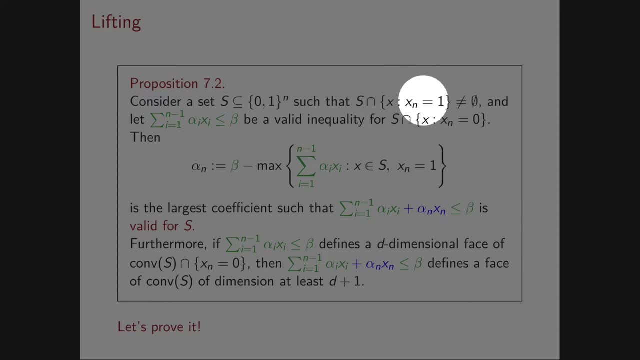 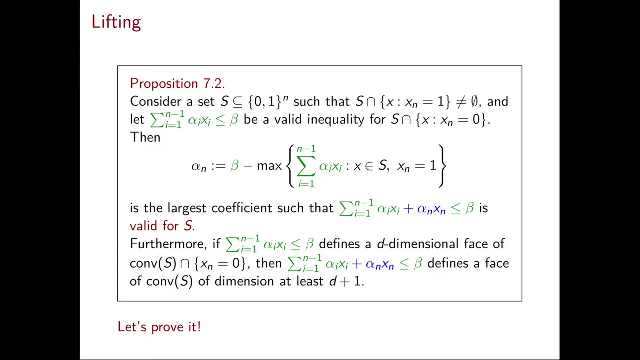 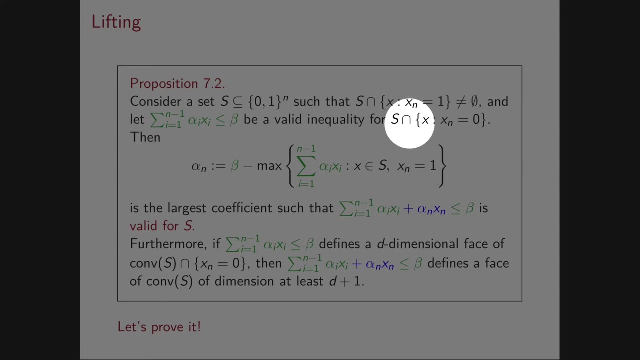 s contains at least a point with xn equal to 1.. In this proposition, we have an inequality whose left hand depends only on the first n minus 1 variables, and it is assumed to be valid for all the points in s with xn equal to 0.. 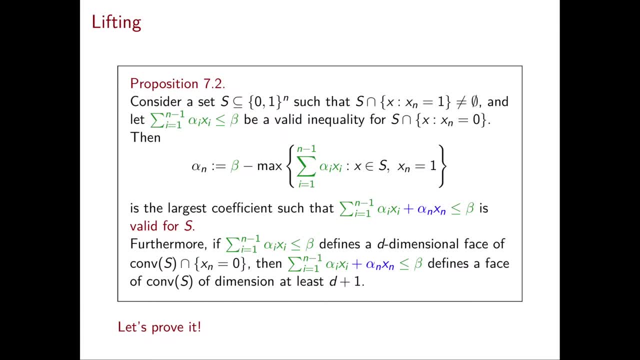 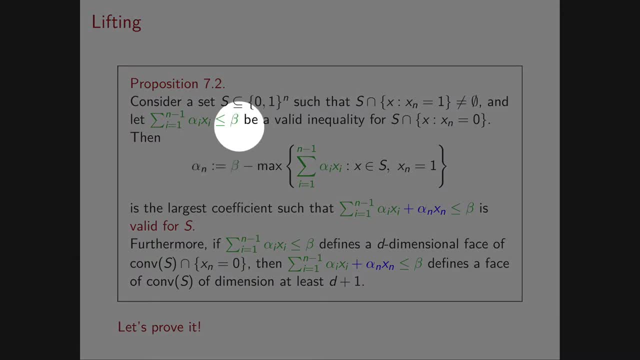 Then we want to find this lifting coefficient, alpha n, and we also want to find the best one. So we define alpha n to be beta. so the original right hand of the inequality minus the max of the original left hand over all points in s with xn equal to 1.. 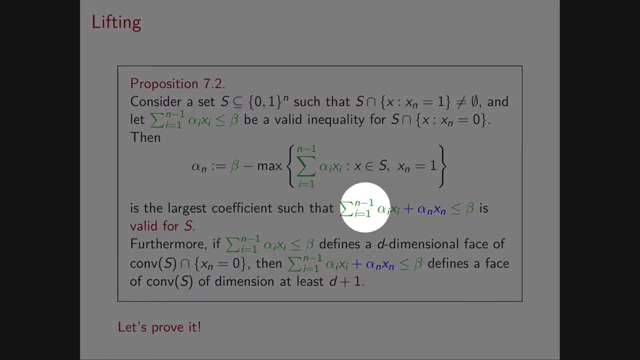 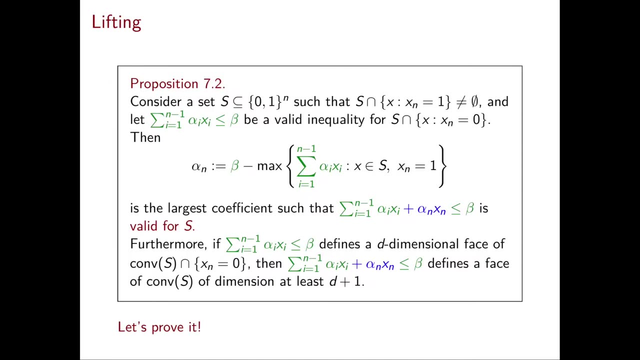 And this alpha n is the largest coefficient, such that the lifting obtained from the original green inequality by adding alpha n, Xn on the left hand is valid for s. The fact that this alpha n is the largest coefficient that gives you a lifting of the green inequality implies the following property: If the original inequality defines the d-dimension, 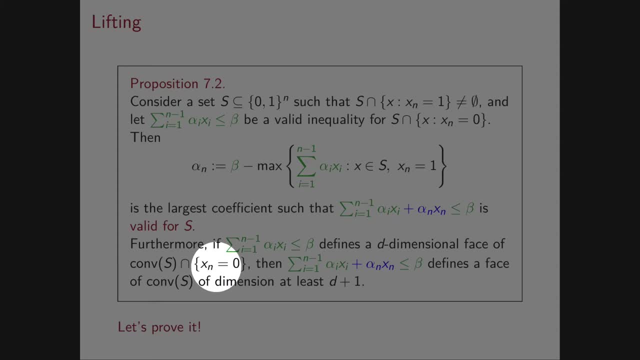 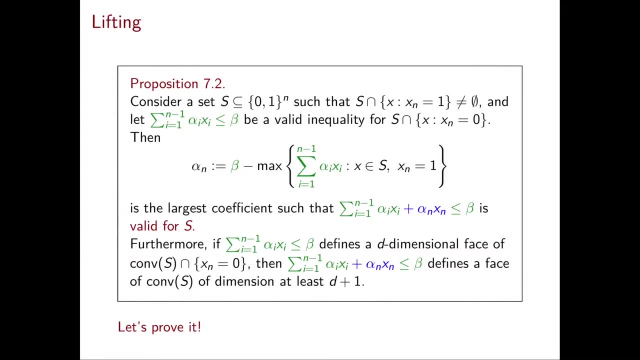 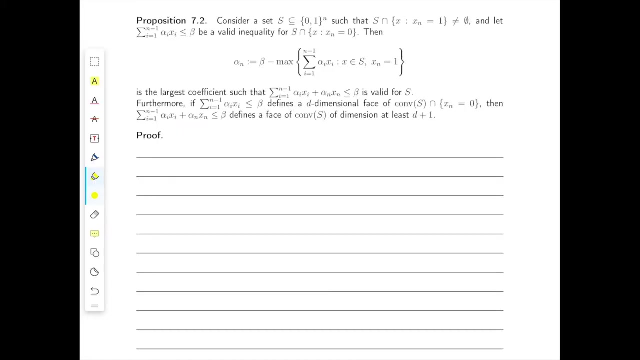 phase of conv s intersected xn equal to 0, then the lifting defines a phase of conv s of dimension at least d plus 1.. Now let's prove this proposition. This proposition asks us to prove a number of things, so let's start by. 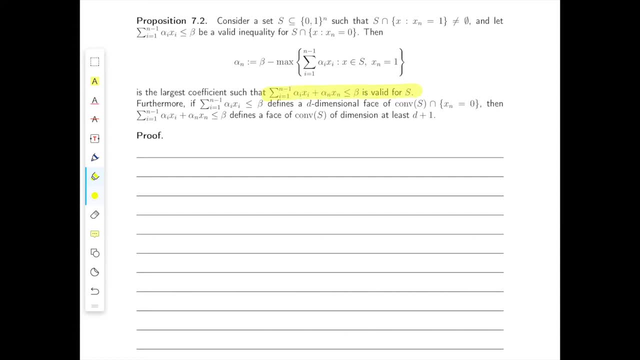 showing that the lifted inequality is valid for s. So to prove that it's valid for s, we prove separately that it's valid for all the points in s with xn equal to 0, and then for all the points in s with xn equal to 1.. So the simpler. 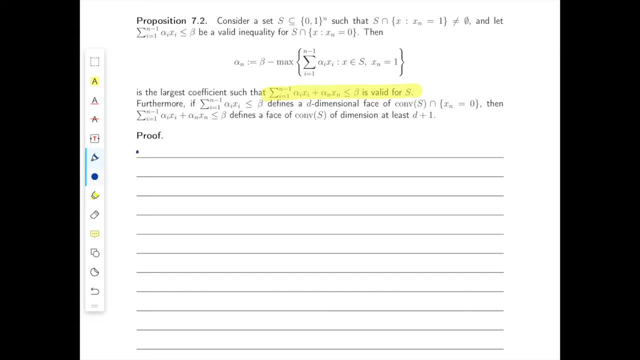 one is for the points with xn equal to 0, because we know this by assumption, Let's write it Great. What about instead the points with xn equal to 1?? So the sum for i that goes from 1 to n of alpha i xi less than or equal to beta is valid for. 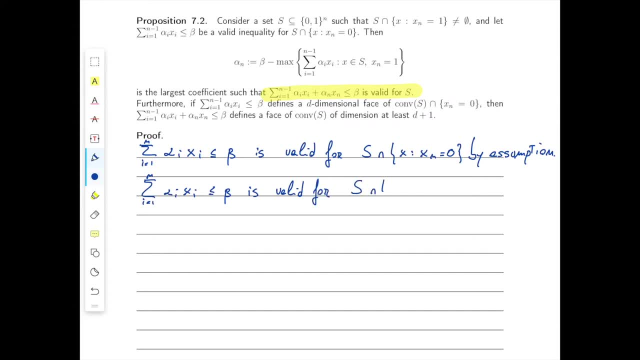 xn. So the sum for i that goes from 1 to n of alpha i, xi less than or equal to beta, is valid for xn equal to 0.. The points in s with xn equal to 1 because for every vector x bar in such a set. 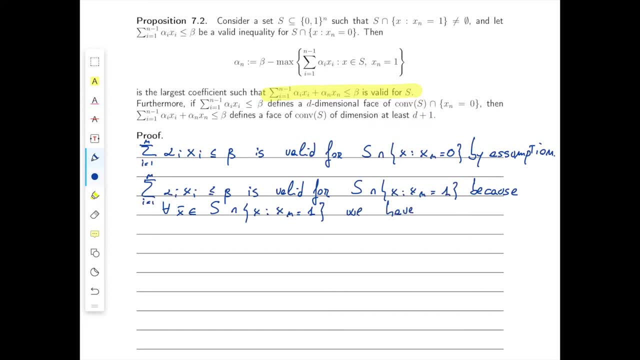 we have sum of alpha i x bar i for i that goes from 1 to n of alpha i xi less than or equal to beta. So let's break this down into the first n minus 1 components and the very last one. So this is the sum for i, equal 1 until n minus 1 of alpha i x bar i plus alpha n times x. 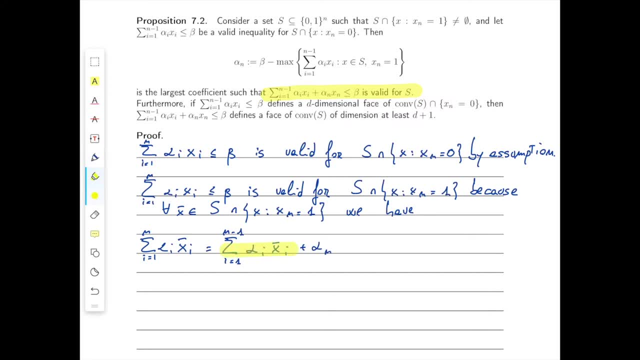 bar n, which is equal to 1.. Now we can upper bound this sum by the max in the definition of alpha n. So the most important, important factor in this sponge is this mx magic Universe. It says xin xn, or equal to the max of the sum, for i equal 1 until n minus 1.. 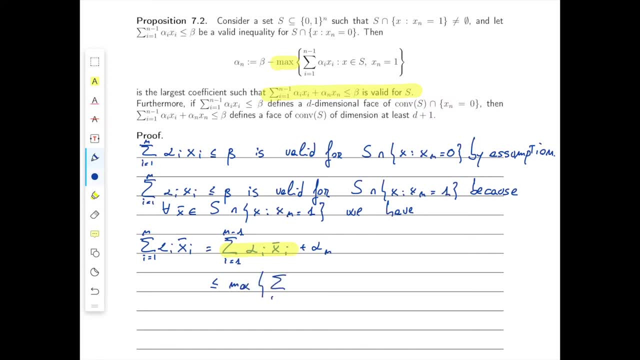 In other words, the sum for alpha i xi less than or equal to the max for i equal 1, until n minus 1 of alpha i xi, such that xxn equal to 1.. This is exactly because the point x bar is indeed in s and has x bar n equal to 1 and. 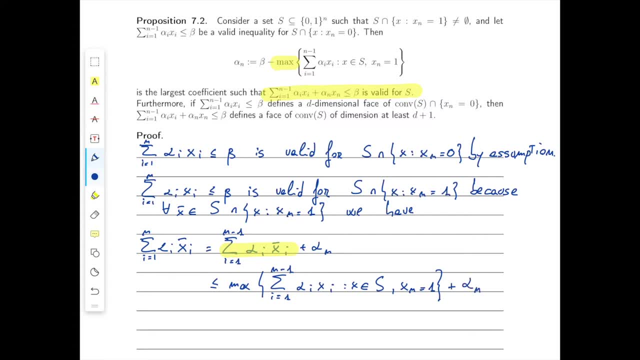 we shouldn't forget plus alpha n At this point. and there's one other weights that we can use for this case. It's stays same as this vertex here, For for local discourse, for here the mx equals 1 and say of alpha n minus 1 times x bar. 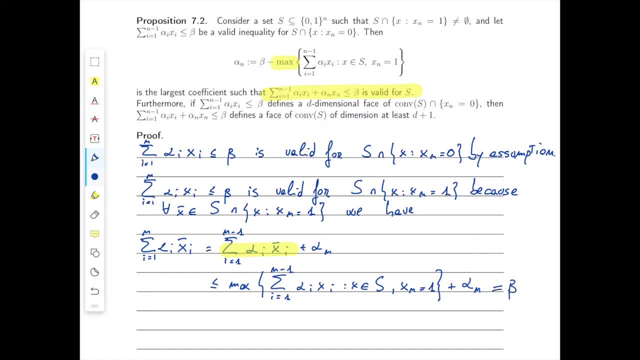 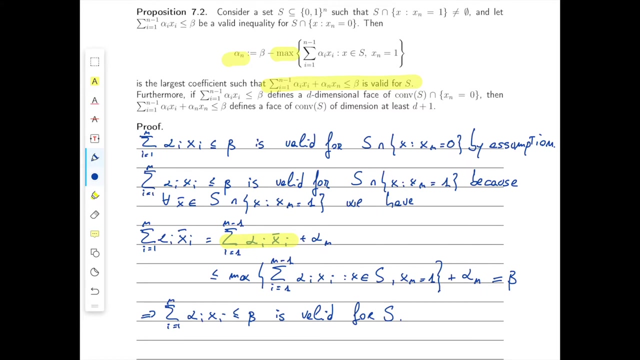 beta from the definition of alpha n in the statement of our proposition. therefore, we have shown that the sum for i equal 1 until n of alpha i, xi less than or equal to beta is valid for capital S. great, so this is the first thing we wanted to show. now let's prove that alpha n is the largest coefficient. 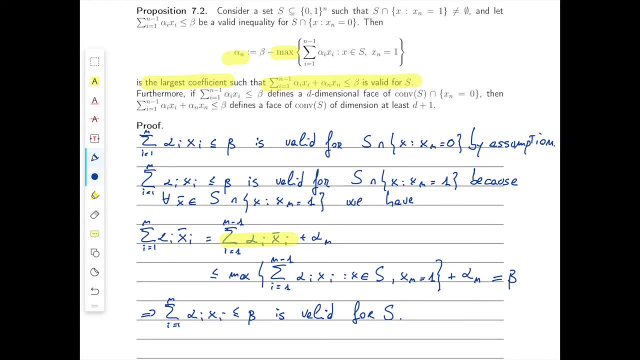 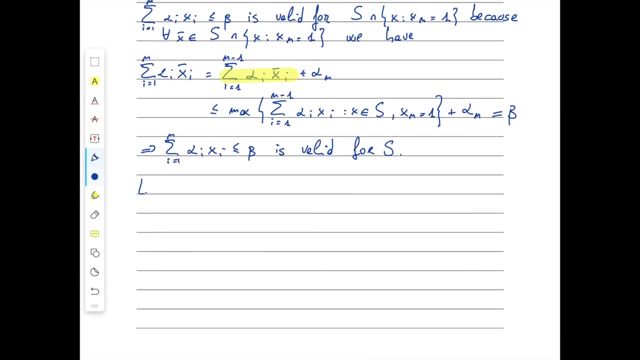 with this property. in order to prove this, we show that the vector x star that achieves the maximum satisfies our lifted inequality at equality. let's write here: let x star in capital S achieving the max, then x star satisfies x star n equal to 1, and we have that the sum for i equal to 1 until n of alpha i. 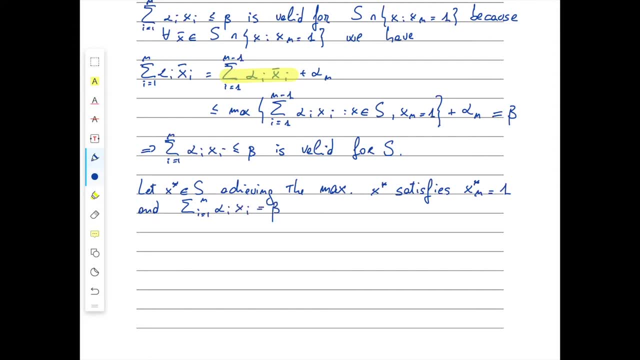 xi, equal to beta. why is that? well, you can go through the chain of inequalities that we just obtained above them and see that, instead of having less than or equal to, we have 춤 deltas menos no I equ- jewelry equality- and so recover quality throughout, and that's how you obtain. 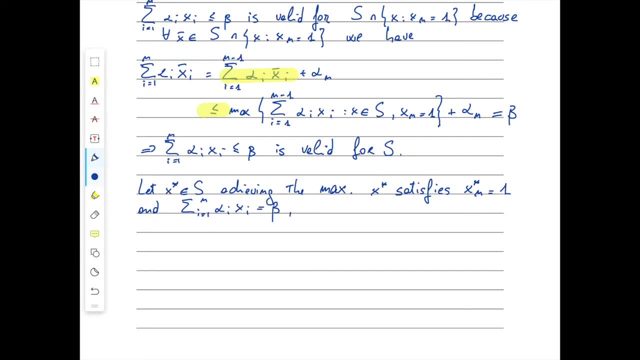 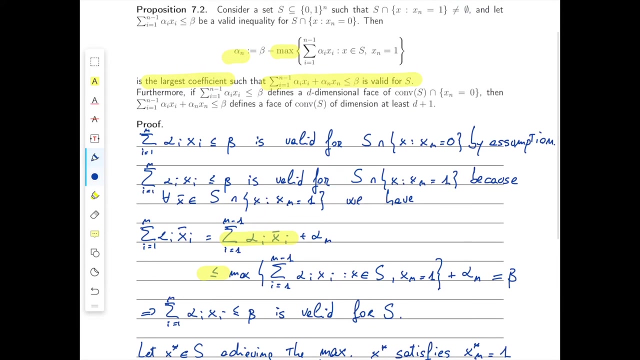 equality S alpha mind. he's the largest efficient ым viewer. we search professor is gonna slow down localization. know already which we should be doing. let's property Great. So now we've shown this part of the proposition as well. Everything we need to show now is about the dimension of the phase. 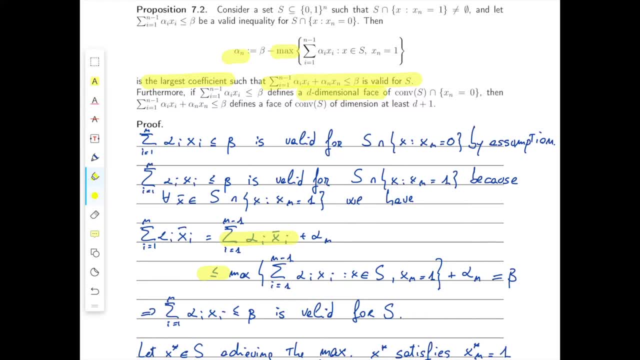 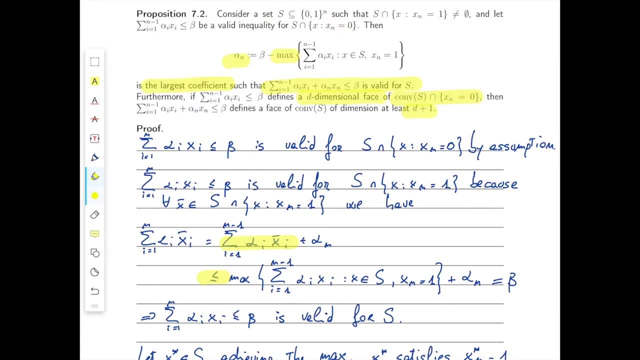 So we're assuming that the original inequality defines a d-dimensional phase of converse, intersected xn equal to zero, And we want to show that the lifted inequality defines a phase of converse of dimension at least d plus one. So this dimension increases by at least one. How are we going to show this? Well, we pick d plus one, a finely independent. 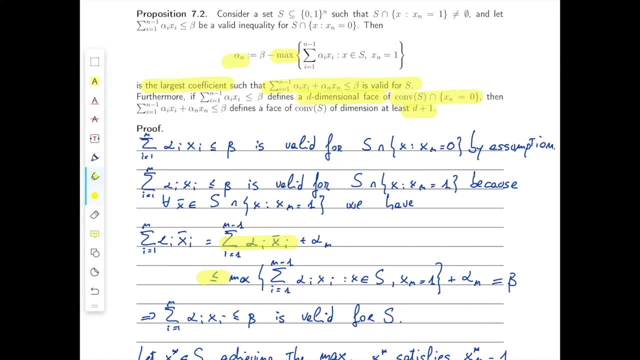 vector in the set converse intersected xn equal to zero, satisfied at equality by the original inequality. Clearly they satisfy at equality also, the lifted inequality, and we just need one more point. And this one more point is exactly our x star. So let's. 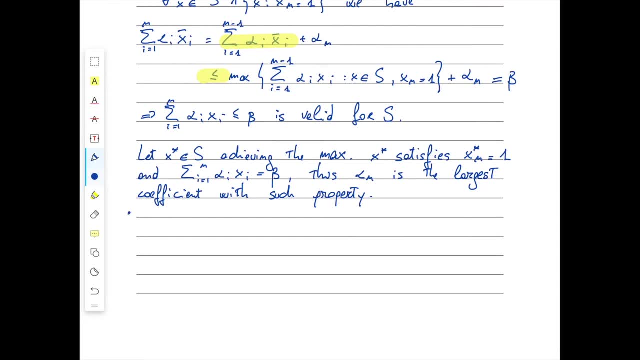 write this. Let's write this down. Consider d plus one, a finely independent point. in converse, intersected x with xn equal to zero, Satisfying For i equal one, until n minus one of alpha i, xi equal to beta, These points also satisfy. 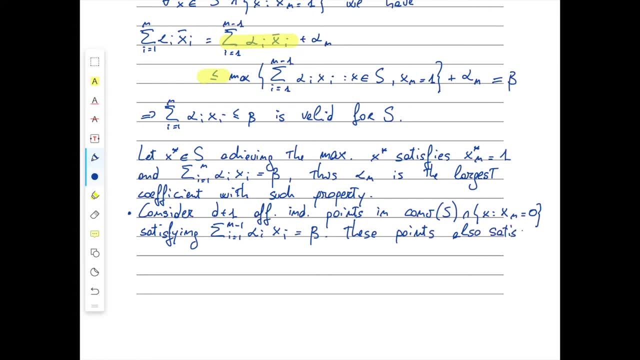 the lifted inequality sum for i equal one until n of alpha i, xi equal to beta. Then we said we want to consider the vector x. The vector x star is a finely independent of the previous d plus one, And this is clear. That's because x star n equal to one, while all the other points have xn equal to zero. 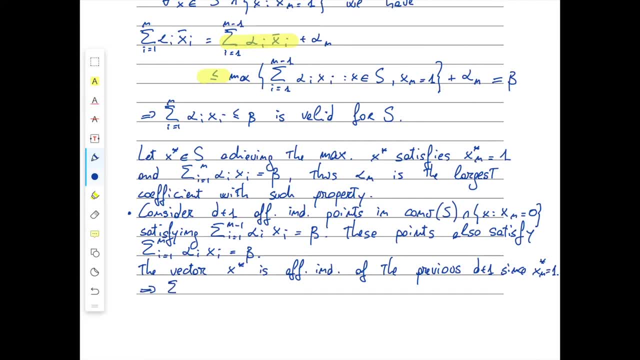 Therefore the lifted inequality sum for i equal one until n of alpha i xi less than or equal to beta, defines a phase of converse of dimension, at least d plus one. And that's it. We've proven everything the propositions had. Let's get back to the slides. 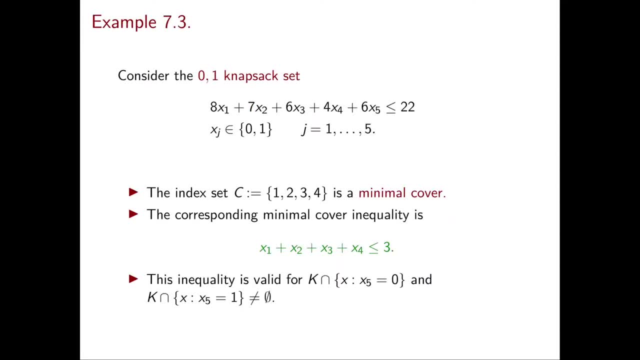 Now that we've understood our lifting proposition, let's look at an example. So let's get back to knapsack sets. Here we have a five dimensional knapsack set. We have binary variables, of course, And this one is our knapsack: inequality. 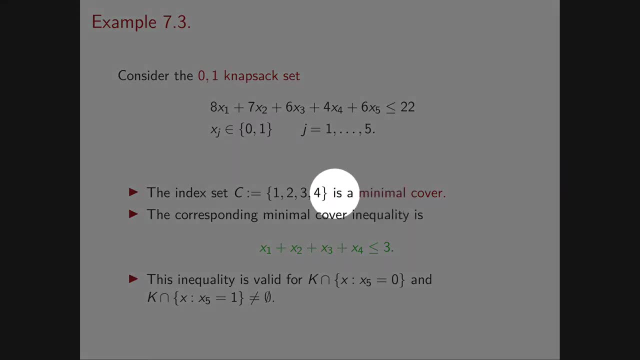 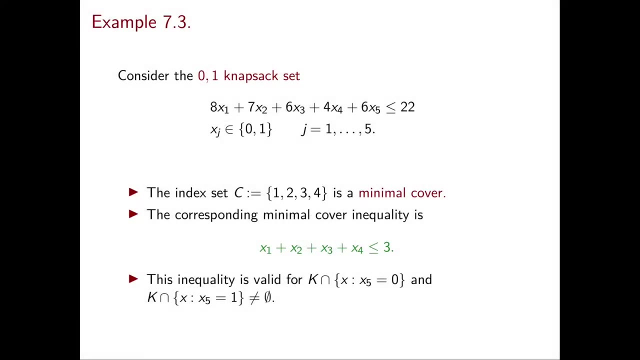 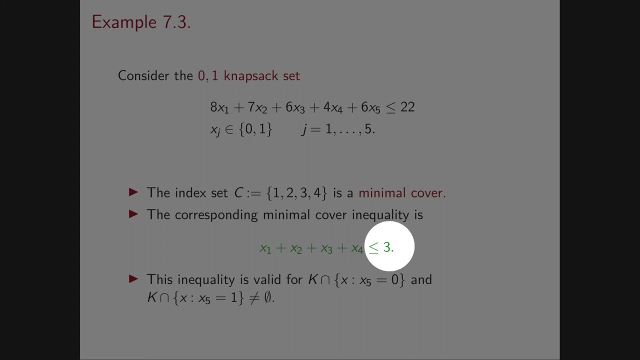 Now let's pick a minimal cover for this set And we claim that one, two, three, four is indeed a minimal cover, And you can check that The minimum cover inequality is x1 plus x2 plus x3 plus x4, at most four minus one. therefore, 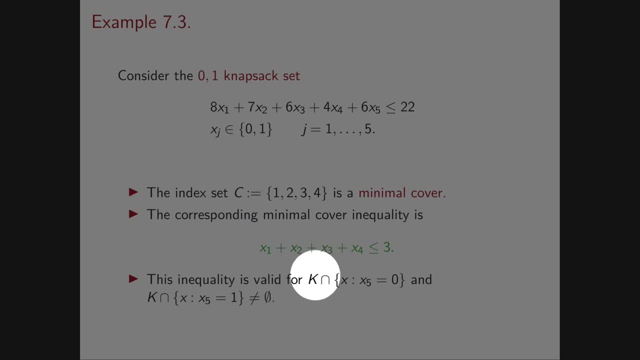 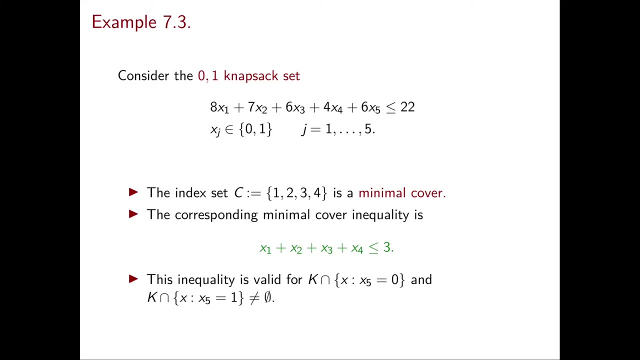 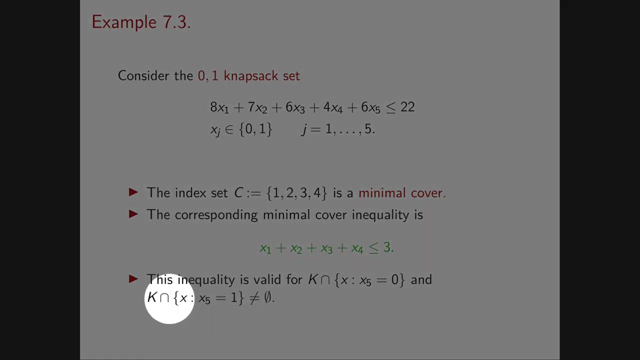 three, We know that minimal cover inequalities are valid for k, So in particular, they are also valid for the phase of k defined by x5 equal to zero. In order to proceed with our proposition, we need to check the technical condition, So we need to see if k intersected x5 equal. 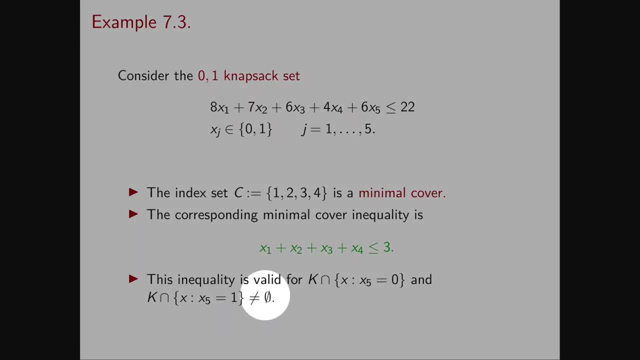 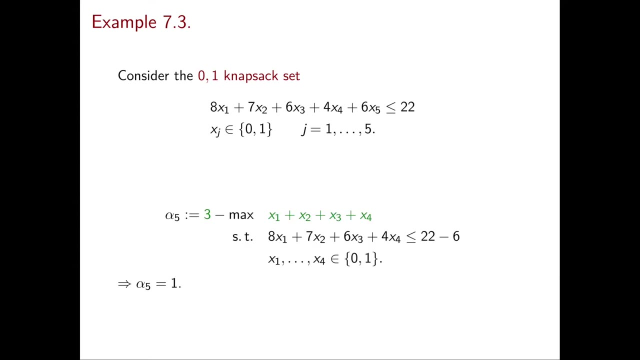 to one. And surely enough it is, because if you set x5 to one, even if everything else is at zero, that's a point in k. Great. So we can then compute alpha five, as the proposition tells us. So we pick the. 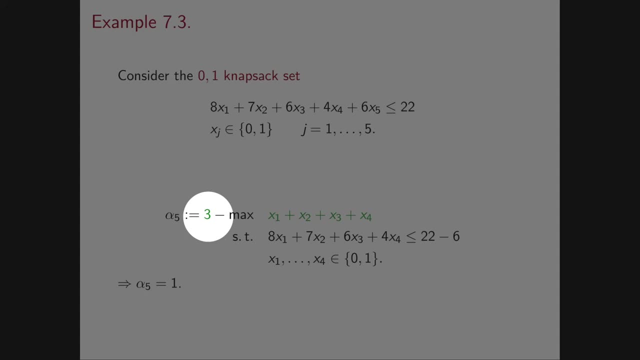 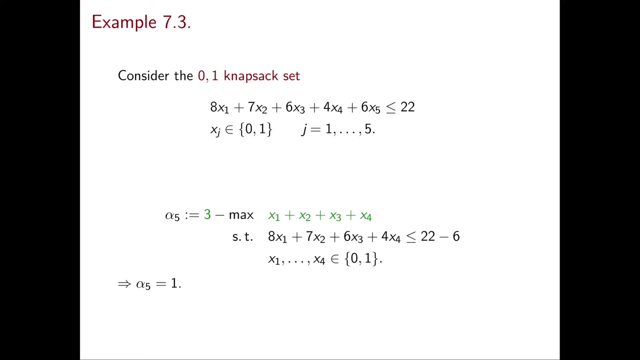 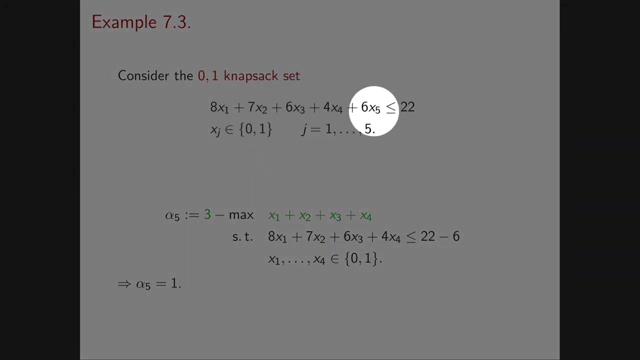 right hand of our original minimal cover inequalities minus the max of the left hand of the inequality, such that the feasible region of the problem in the proposition is the original feasible region, but where we set, in this case, x5 to one. So we have 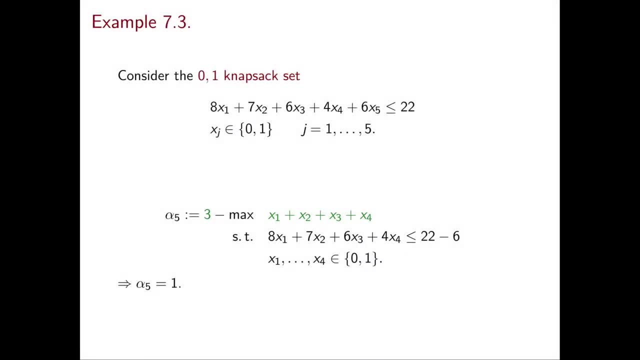 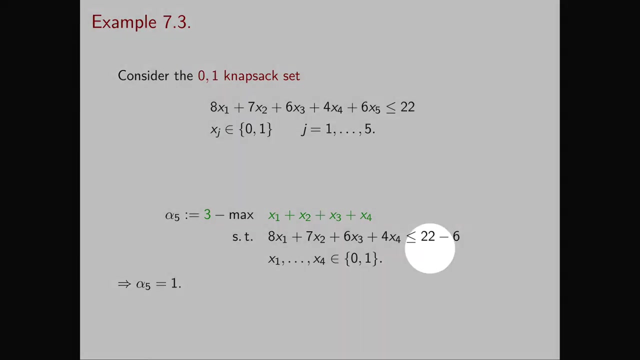 the same inequality until four x four, But then we have, plus six, less than or equal to twenty two. Therefore, if we bring the constants to the right hand, we have that the left hand is less than or equal to twenty two minus six. In particular, this is a four-dimensional. 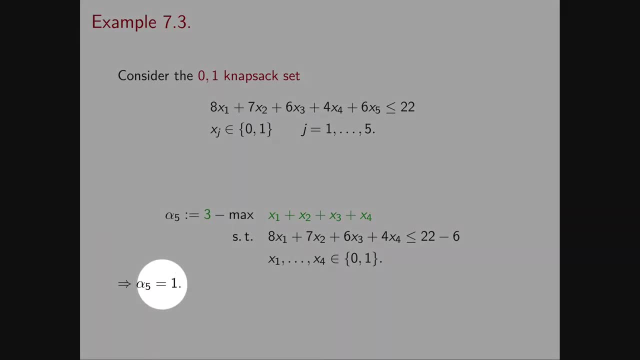 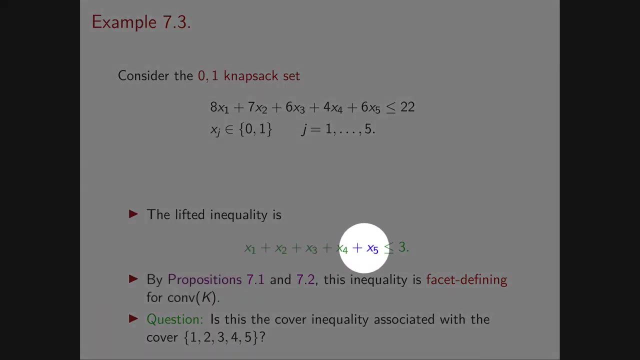 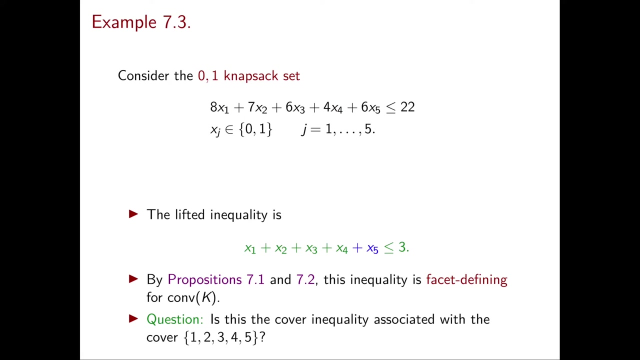 integer programming problem And if you solve it you obtain that alpha five is equal to 1. therefore the lifted inequality is the original green one plus alpha 5, which is 1 times x5 less than or equal to 3, which is the original right hand side In. 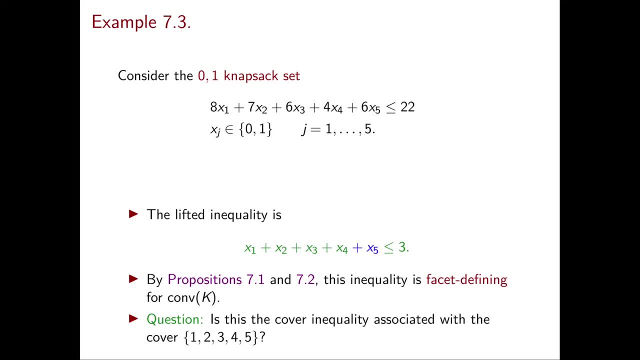 proposition 7.1 we saw that the green inequality is a facet defining for conv k intersected x5 equal to 0. therefore, the proposition 7.2 implies that the lifted inequality is now facet defining for the full conv k. Note that this inequality looks similar to a cover inequality, for example. one could wonder: 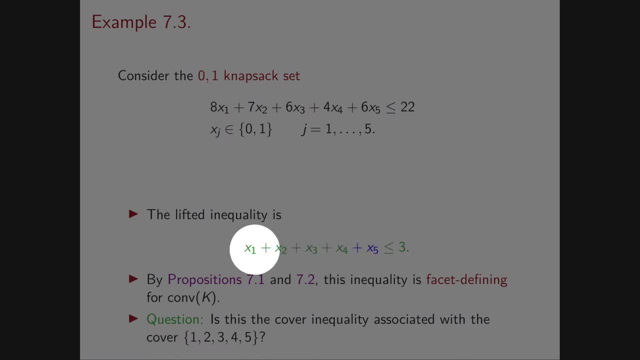 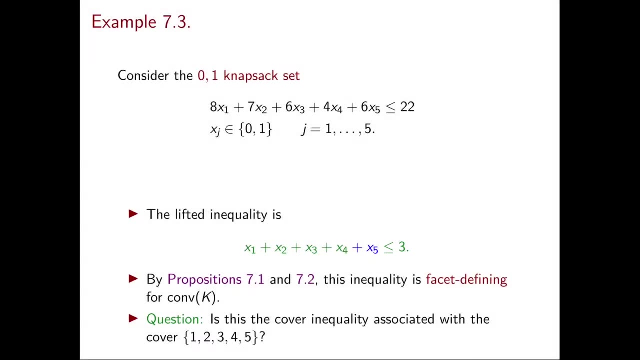 is this the cover inequality associated with a cover from 1 to 5?? Well, of course it's not, because the right hand of such a inequality is the same as the right hand of such a inequality. Therefore, the cover inequality should be 4, so this inequality is much stronger because it's. 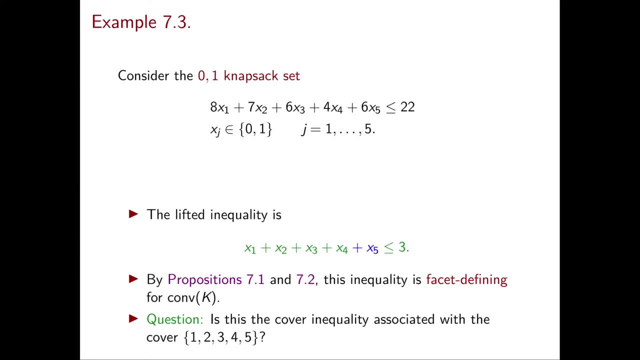 less than or equal to 3, instead of less than or equal to 4.. Great, so in this example, we've understood how to lift a minimal cover inequality for a 0-1 knapsack set. Now the question is: are you able to lift any minimal cover? 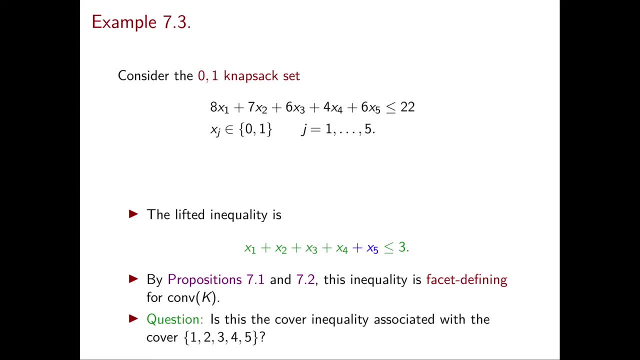 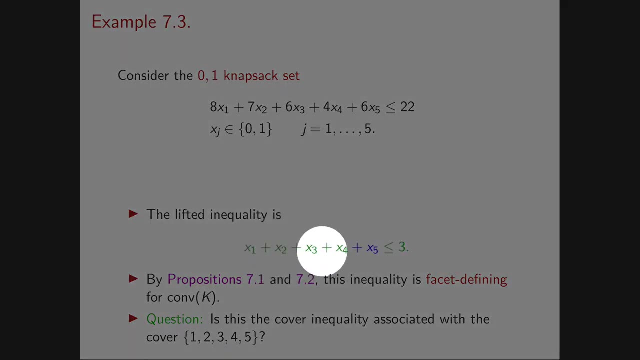 inequalities for 0-1 knapsack sets. Well, not exactly, at least not directly, because this example was chosen in such a way that you can apply directly proposition 7.2.. In fact, the minimal cover inequality contained all the variables until variable n-1 and we lifted the last. 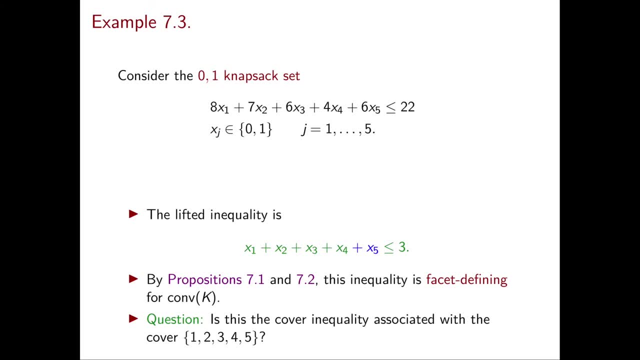 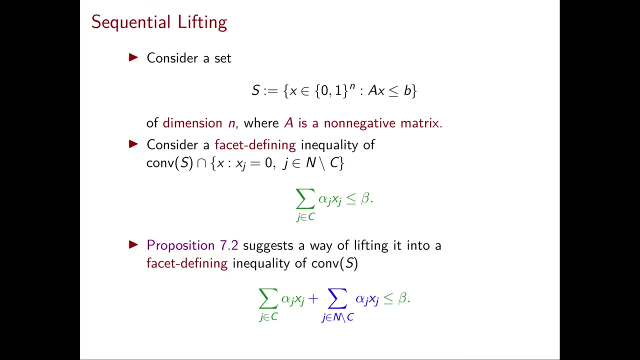 variable. In general, you could have a minimal cover inequalities that contains fewer than n-1 variables on the left hand, And the question is: can we then lift also such inequalities? So let's let's again go to the more general case and answer this question in this more general setting. 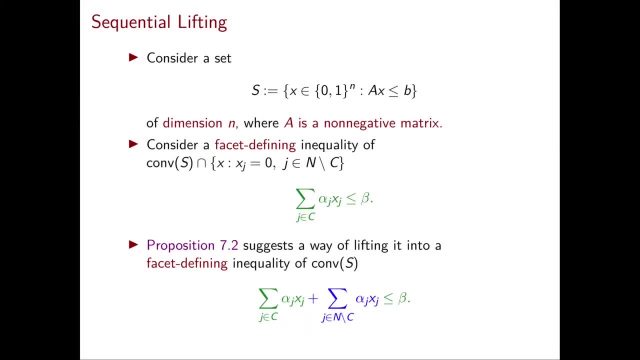 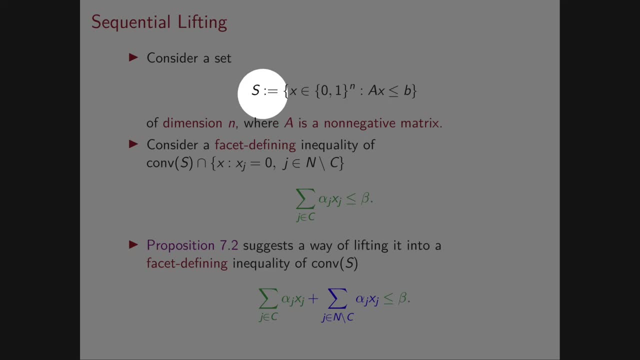 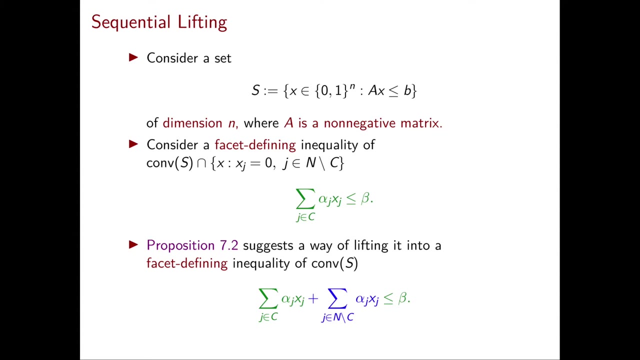 consider a general zero, one linear set, and in this case we need a technical assumption, namely that the matrix a defining the set s is non-negative. we definitely need this assumption, but it's a bit technical at this point so maybe just forget it for now. i'll get back to it. now, assume that 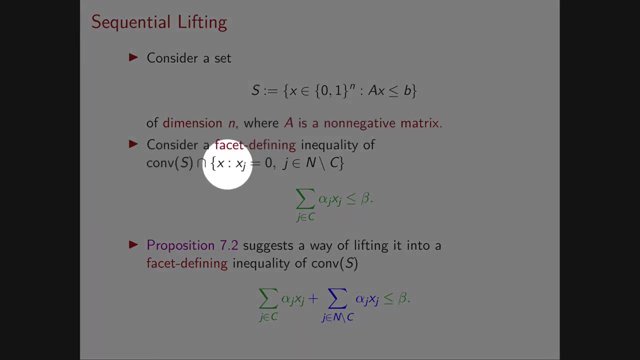 you have a faster defining inequality for converse intersected xj equal to 0, not only for one variable but for a bunch of variables, all the variables in n minus c. and assume that your inequality is exactly of the form sum of alpha, j, x, j for j only in c, less than or equal to beta, and this is exactly. 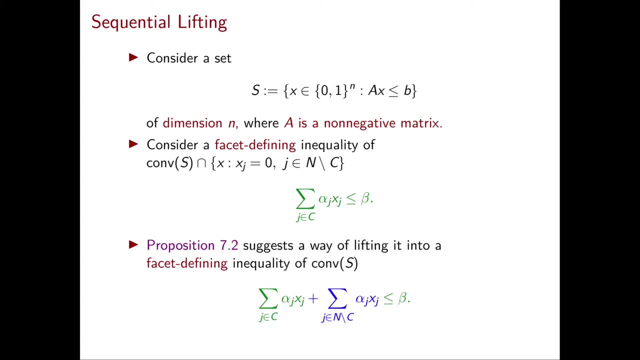 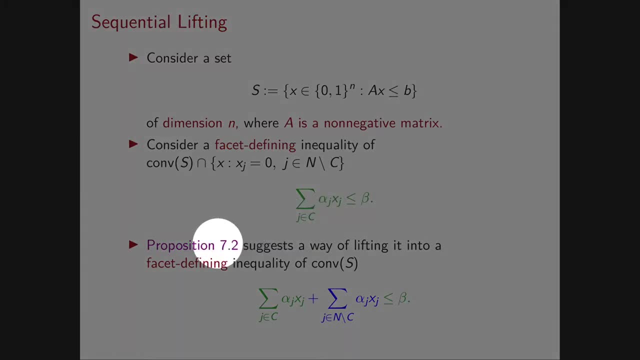 what we have in the case of minimal cover inequalities, as we saw essentially in the first slide of this section. now we can essentially use our lifting proposition to lift this inequality into a faster defining inequality of converse. so what do we need to do? we need to add sum of alpha, j, x, j for every j in n minus c. the fact is that our proposition 7.2. 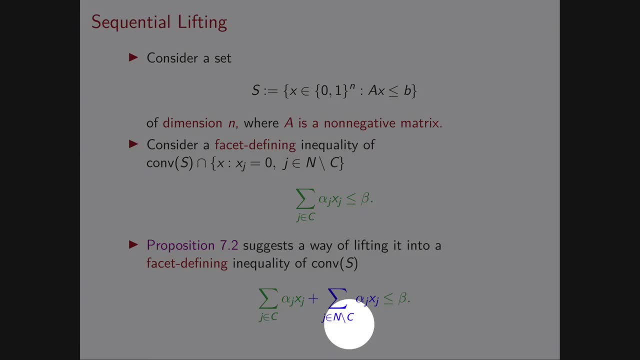 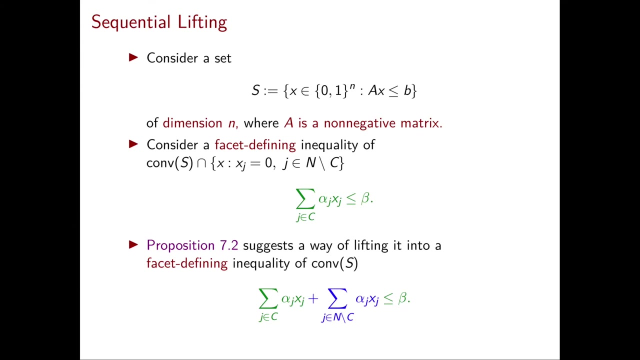 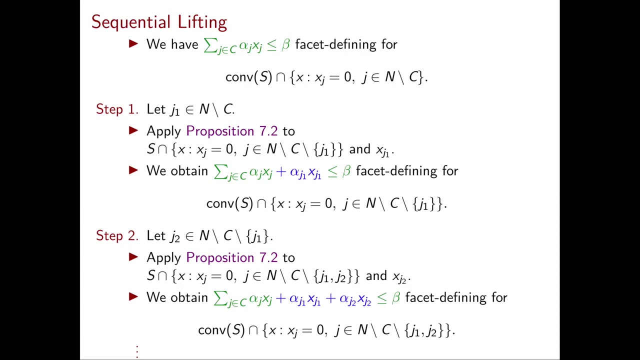 only allows us to add one alpha j, x j at the time. therefore, what we can do is apply the proposition recursively in order to obtain, one by one, this coefficients alpha j. so let's just see explicitly what we want to do. so again, we have our inequality. that is our starting point. as always in green, it's. 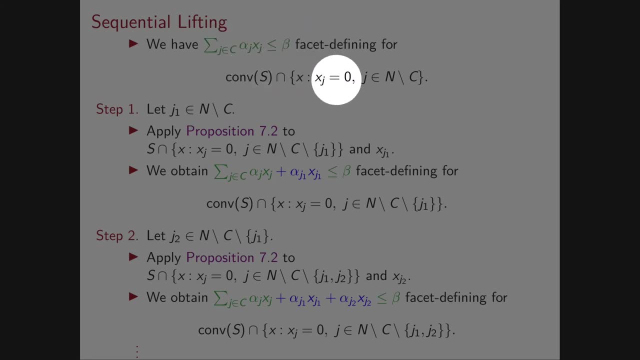 faster defining for again: converse: intersected x j equal to 0 for every j in n minus c. so what we want to do is pick one by one the indices in n minus c and remove them, essentially because we eventually want to obtain an inequality. that is faster defining only for converse. 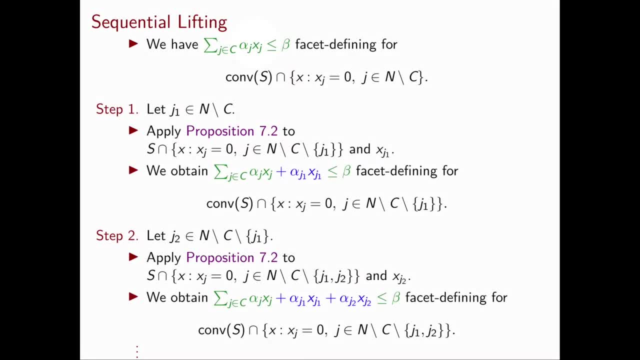 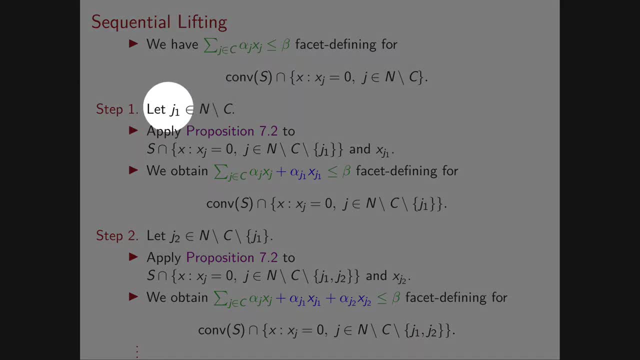 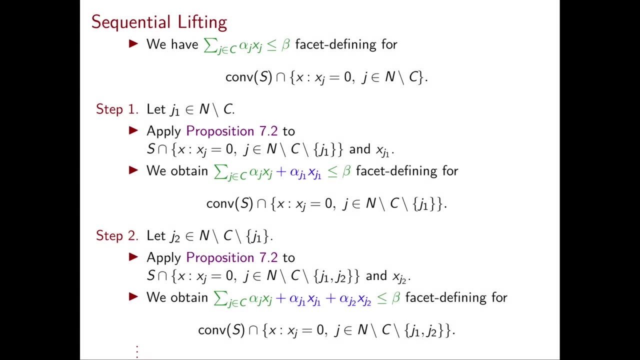 and one by one we want to bring them inside the inequality. so let's pick the first index that we want to bring from here to the inequality. so let j1 be in n minus c. now we apply proposition 7.2. but we have to be a little bit careful to which sets and which variables we apply such a proposition. 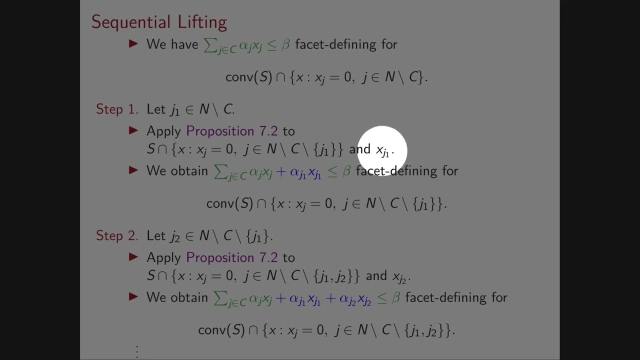 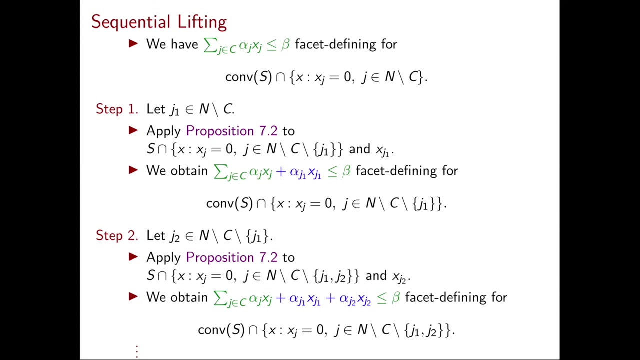 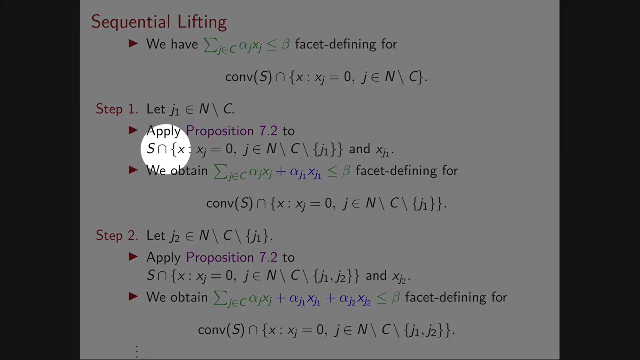 so clearly, the variable that we want to lift is x, j- 1, but then what is the set that we call the capital s inside the proposition? well, this set changes essentially at every iteration. here, in our first iteration, the one we're discussing now, we need to consider the set s intersected: x, j equal to 0, for 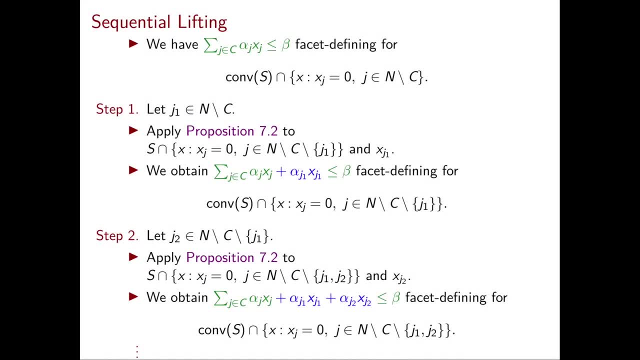 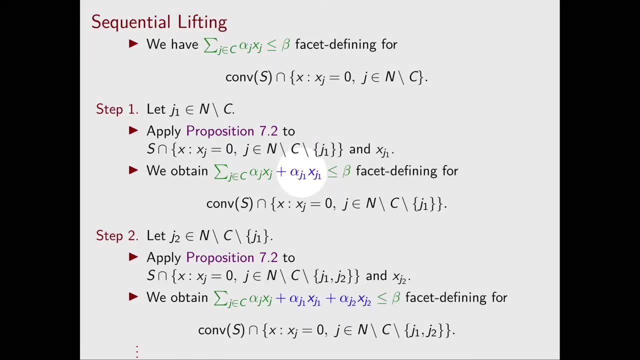 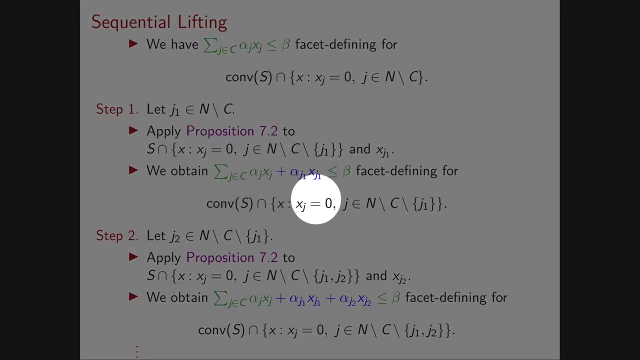 every j in n minus c minus j 1. in this way, if we apply the proposition, we obtain a lifting of the gradient inequality where we also have alpha y, the result of a linear select graph, which We also have alpha j1, x, j1, and it is a facet defining for conv s intersected now x, j equal to 0 for j in n minus c minus j1.. 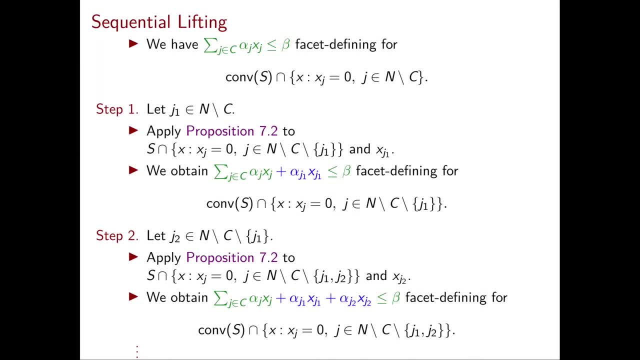 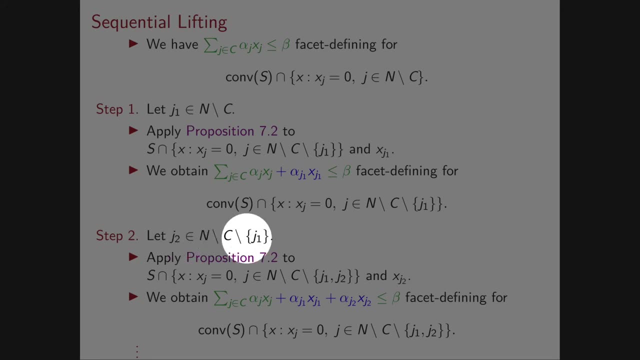 So this is a larger set than the one before, and we're working our way towards having just conv? s here. In the second step we take a j2. now it has to be in n minus c, but also minus j1, because now j1 has been lifted already. 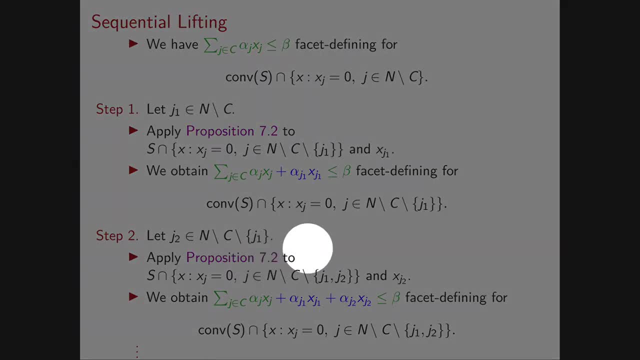 And now we apply again the proposition 7.2. we want to lift x, j2 and the set in the proposition must be s intersected x j, equal to 0 for every j in n minus c minus j1 j2.. And again due to the proposition, we are also able now to lift. 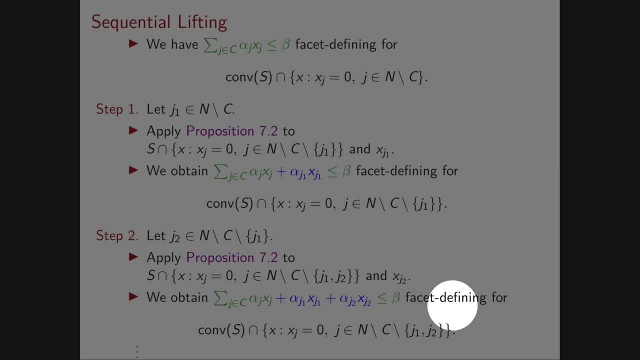 So we have a facet defining for conv s intersected now x- j equal to 0 for j in n minus c minus j1 j2.. The second variable and we obtain a facet defining inequality for conv s with x- j equal to 0 for every j in n minus c minus j1 j2.. 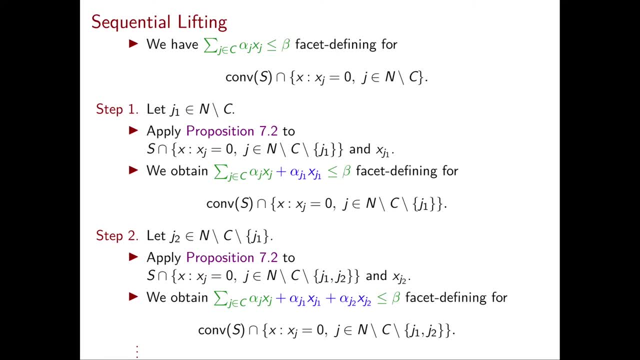 And so on and so forth. if you continue until you have considered all the indices in n minus c, you will end up with a facet defining inequality for the set conv? s. So let's see now, algorithmically, what we have to do in order to perform this sequential lifting. 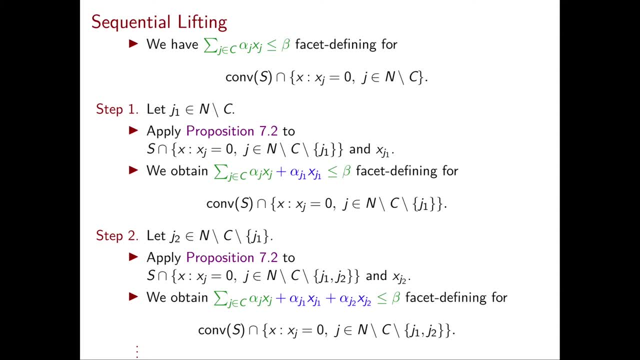 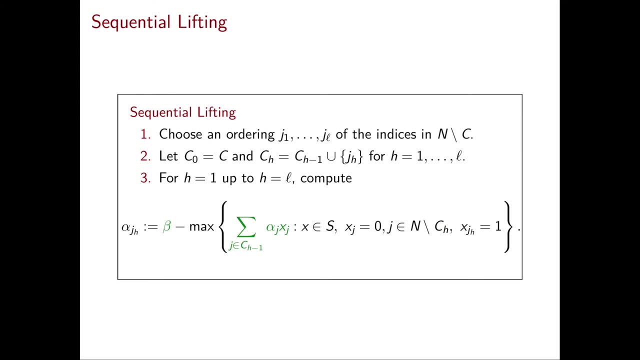 In fact, In this discussion I didn't even write exactly how to compute the coefficients alpha, j, i. So in sequential lifting, the first step consists in choosing an ordering of all the indices that we have to lift, those in n minus c. Next it will be useful to define the sets c- h such that at iteration age, c- h contains the indices of the variables that appear in the inequality. 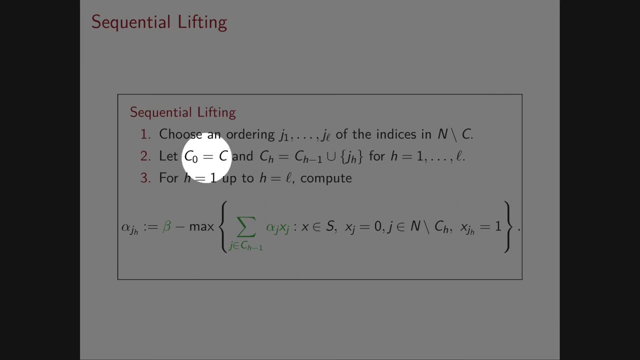 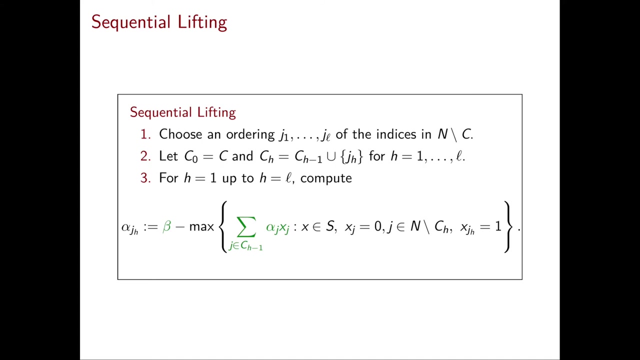 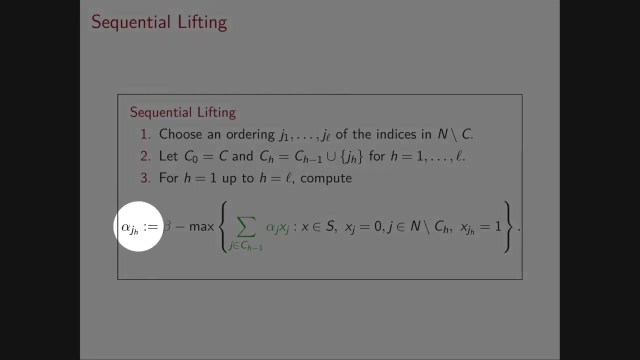 So at the beginning or the 0th iteration, we have c0, equal to c, and then one by one, we add the j age in exactly the order that we pick them. Now we're only left with the question: how should you calculate alpha j h? and for this we just need to apply the proposition we have that alpha j h is beta. this never changes. is the original right hand. 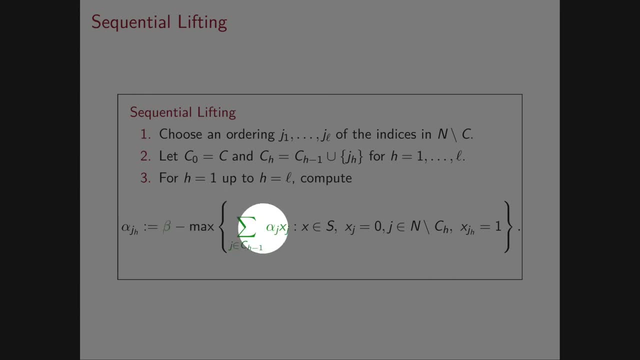 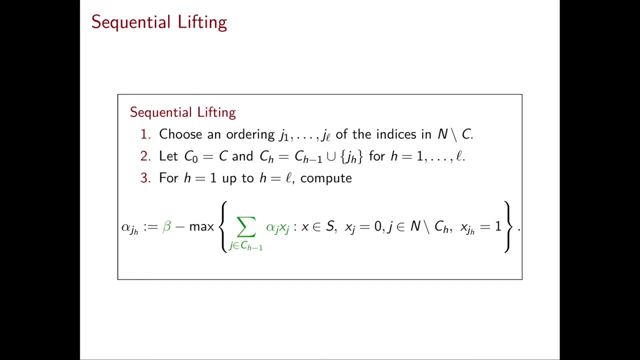 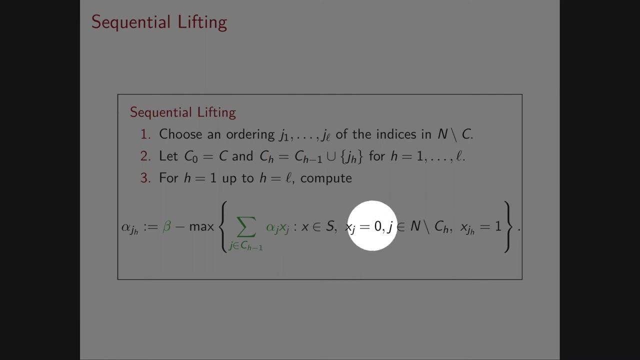 minus the max of The sum of alpha, j, x, j for j in c, h minus one, and this is the left hand side of the lifted inequality obtained so far, Such that x is in s and x, j is zero for every j in n minus c, h and x, j, h, equal to one. 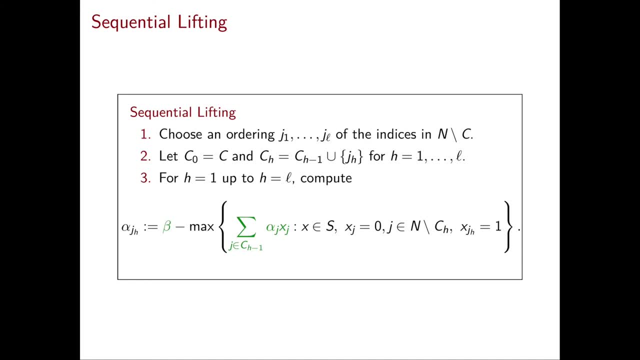 At this point. if you remember, a couple of slides ago, we made t equal to one And then we had the following expression: We made t equal to one, and so on. So for each j in n minus c, h, we add the x, j, h equal to one, and so on. 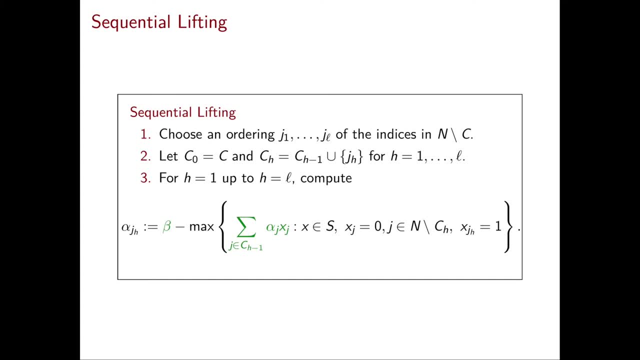 technical assumption that our set S has dimension n and defined by a matrix that is non-negative. and the question is: why did we need those technical assumptions? and the answer is: we need these assumptions in order to apply proposition 7.2. in fact, if you remember, in order to apply such a proposition, we 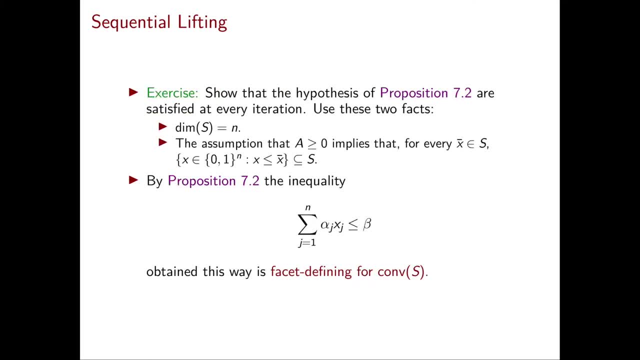 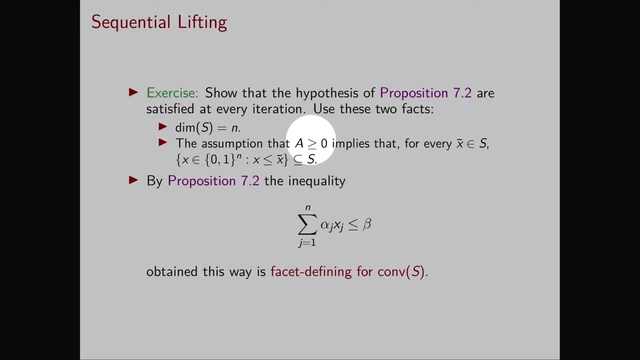 need to check a couple of conditions, and it's a very good exercise to check that, in fact, the hypotheses of the proposition are satisfied at each iteration. and that's exactly where you need to use our assumptions that the dimension of S is n and that a is greater than or equal to 0, in particular, 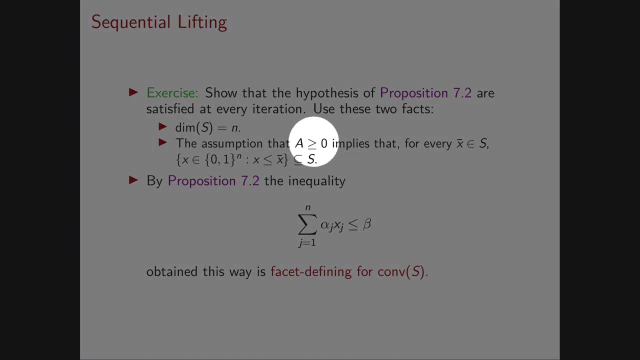 you need this- a greater than or equal to 0- to show that for every point in S, then also all the points that are binary and with X upper bounded by X bar are contained in S as well. once you've checked that the hypothesis is correct and you've seen that you can add the functions to the. 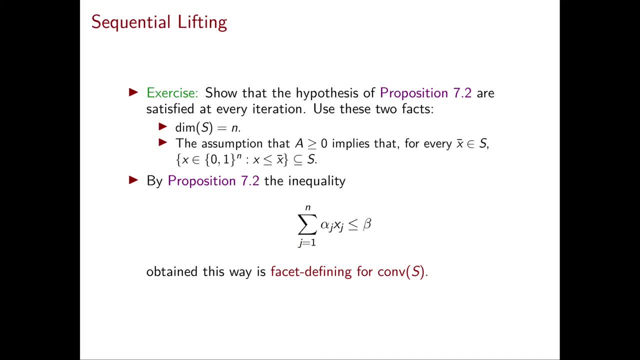 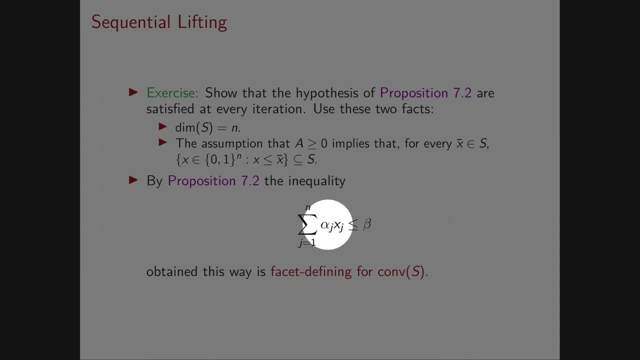 of proposition 7.2 are always satisfied, then. indeed, proposition 7.2 implies that the full inequality that you obtain at the very end, so the one with all the coefficients, alpha j for j equal to 1 until n at the very end, is a facet. 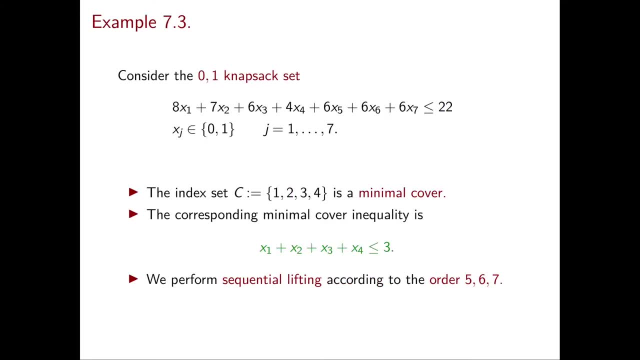 defining for the convex hull of S. Let's see an example of sequential lifting. As always, we look at a 0-1 knapsack. set Here it is. This example is very similar to the previous one. we just have more variables. essentially Now, in fact, it is. 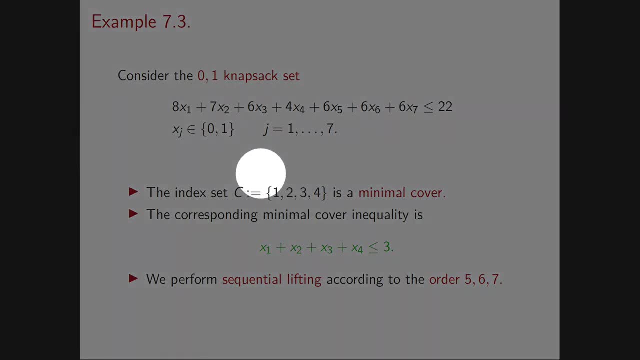 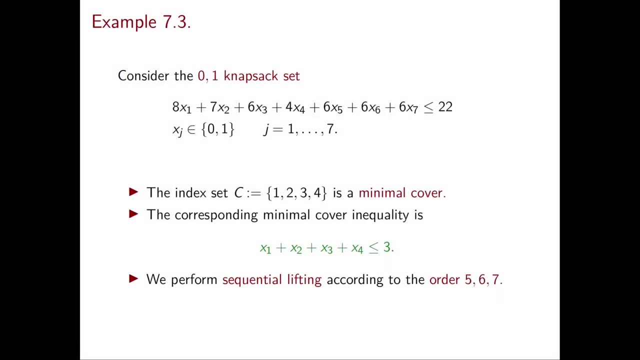 a seven-dimensional problem, As before. 1,, 2,, 3,, 4 is a minimal cover and the corresponding minimal cover inequality is this one in green: x1 plus x2 plus x3 plus x4, less than or equal to 3.. And now we perform sequential lifting according: 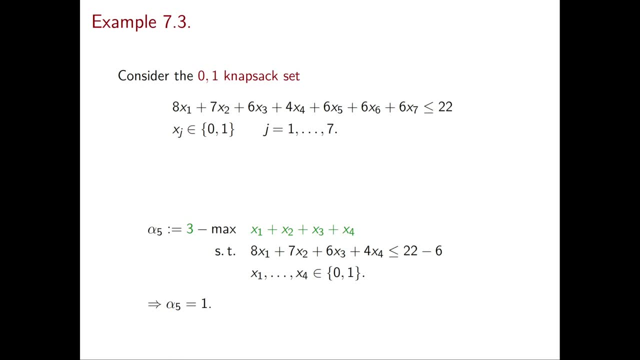 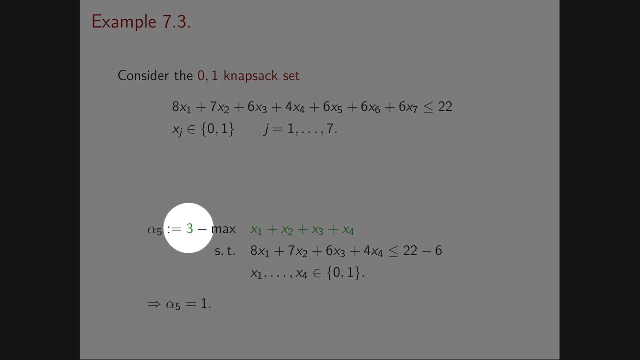 to the order, let's say 5,, 6,, 7.. Therefore, first we want to understand the coefficient alpha j, Alpha 5, and it's defined as right-hand side, so 3 minus max of left-hand side of the inequality Subject 2, so what we need to do is pick the original inequality. 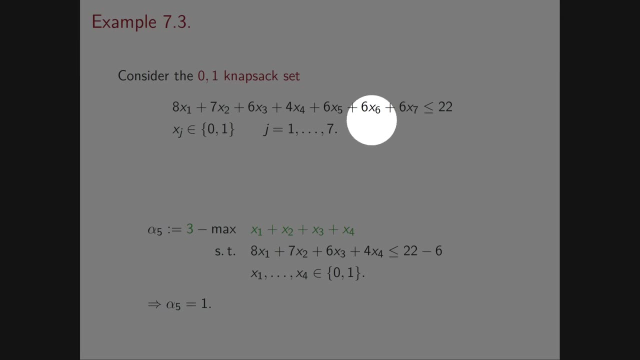 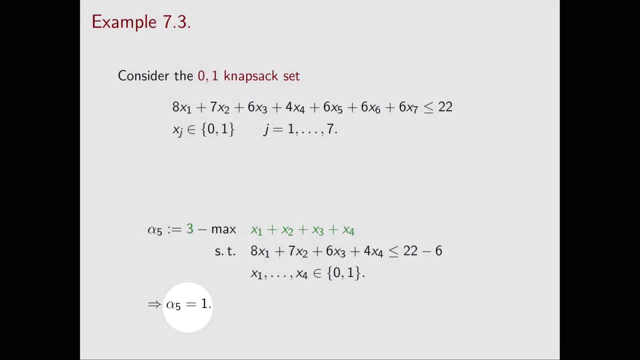 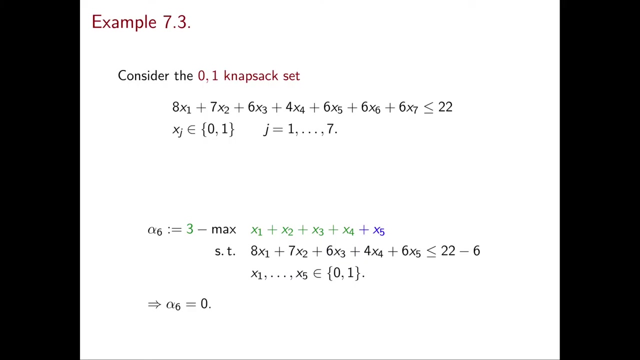 set x6 and x7 to 0 and x5 to 1, and this is the inequality that we obtained. This is a four-dimensional problem and if you solve it, you obtain alpha 5 equal to 1.. Next we want to find alpha 6.. At this point, we're considering the inequality that we 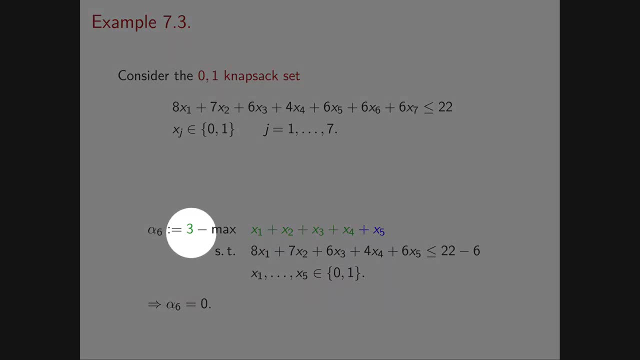 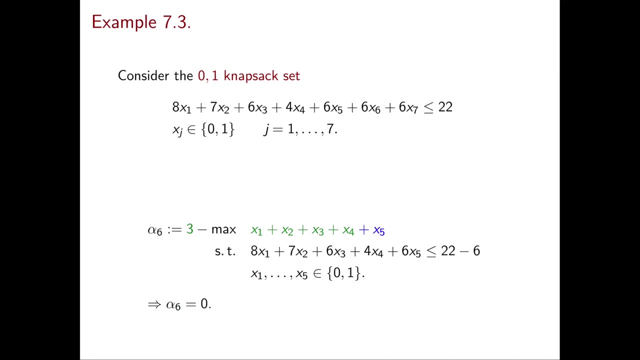 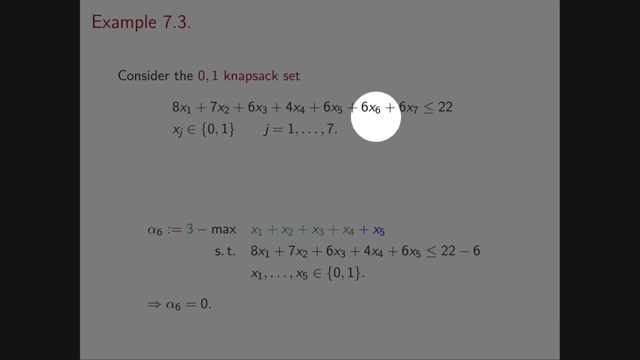 just lifted. So the right-hand side is always the same, it's 3, but then in the max we have the new left-hand side. so we also have a plus alpha 5 x 5, and the constraint is the original constraint, where we set x 7 to 0 and x 6 to 1.. 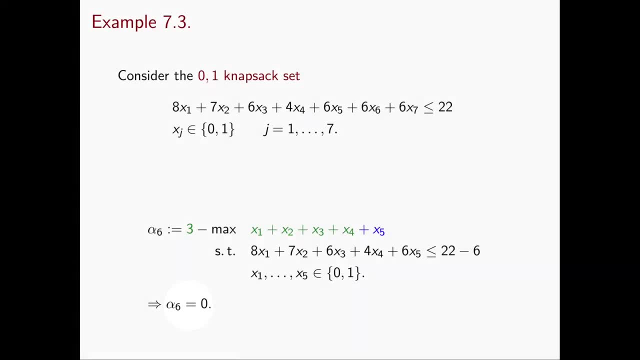 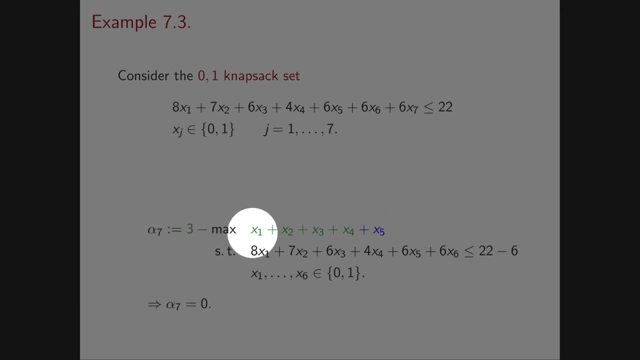 This is a five-dimensional problem and we obtain alpha 6 equal to 0. if we solve it, 7, again 3 minus the max of the current lifting. now we have plus x5, as before, plus alpha 6, x6, which is 0 because we obtained alpha 6 equal to 0. now the inequality is the original one, where we 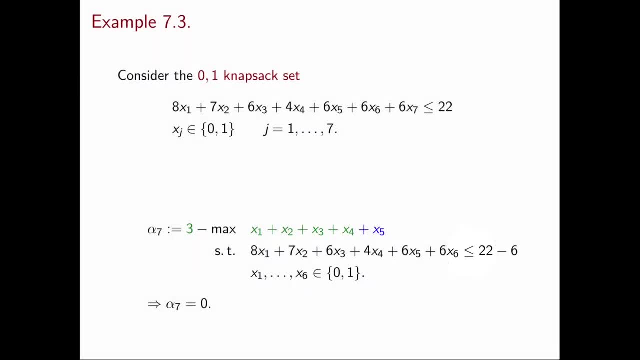 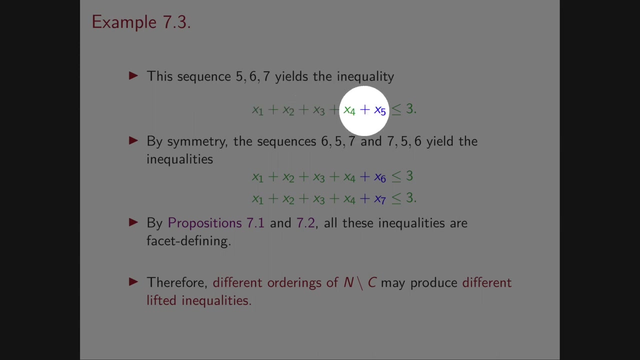 set x7 to 1 and we obtain this inequality. this problem has dimension 6 and if you solve it, you obtain alpha 7 equal to 0. therefore, the final lifted inequality is the following: x1 plus x2 plus x3 plus x4 plus x5, less than or equal to 3- note that our problem was extremely symmetric. 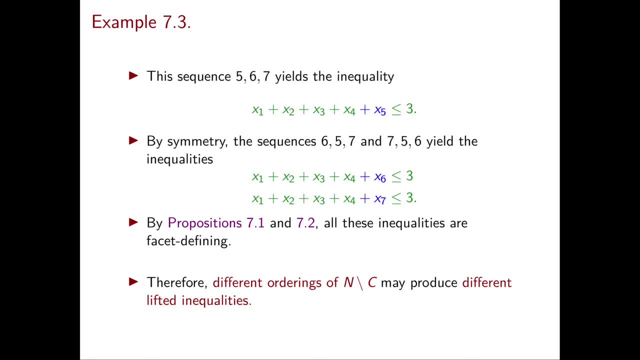 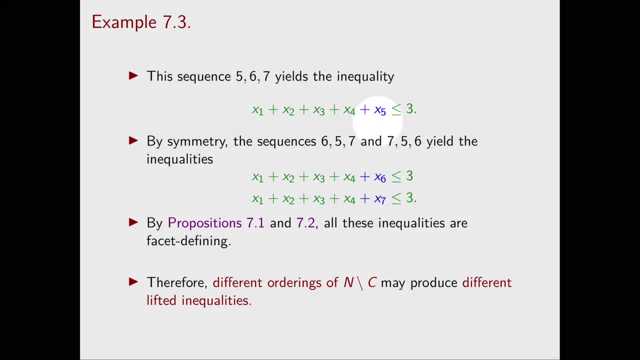 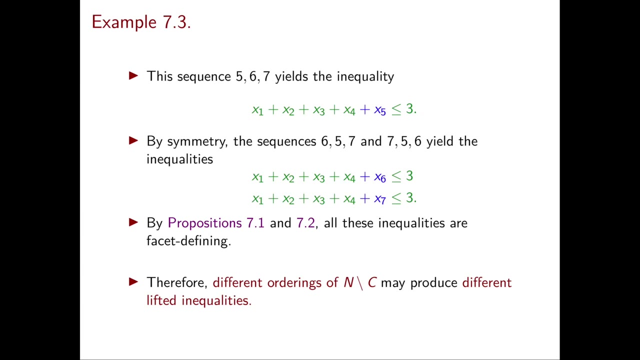 because in the knapsack inequality we had the same weight for x5, x6 and x7 and so by symmetry you can check that if you picked any other order of the variables for the sequential lifting we would have obtained the following inequalities: it's always the first. 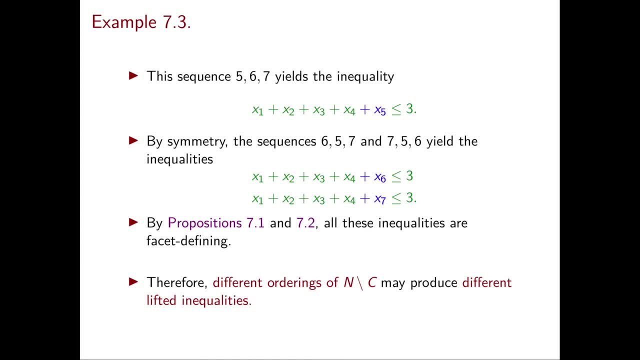 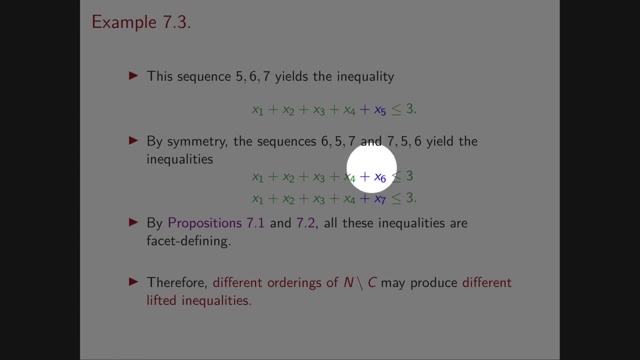 that gets a plus one coefficient, and the second and third, we get a zero coefficient. so you obtain the same inequality as the one we have seen in detail, but with plus x6 and plus x7 instead of plus x5. we know by proposition 7.1 that the original inequality is facet. defining for the 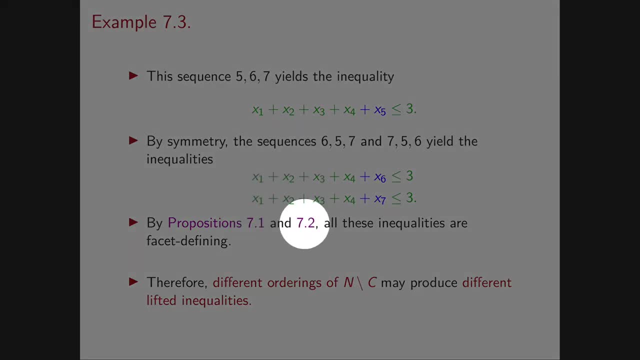 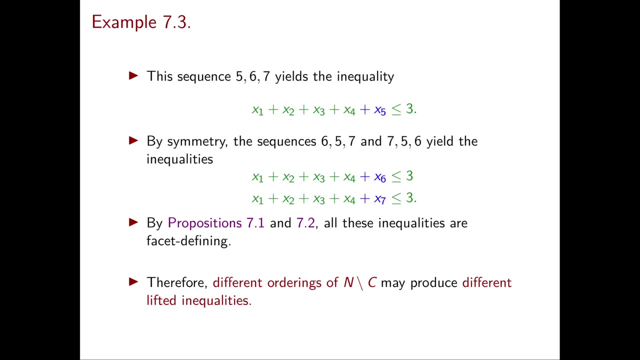 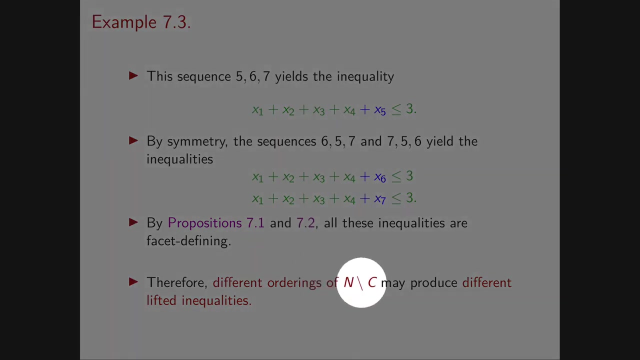 corresponding phase and by proposition 7.2, the inequality obtained at the end of our sequential lifting is facet defining for the full set. so all these inequalities are facet defining for count k in particular. in this example we've understood that if you pick different orderings of the variables to be, 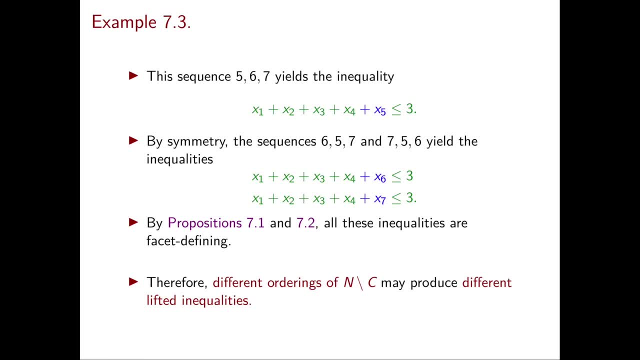 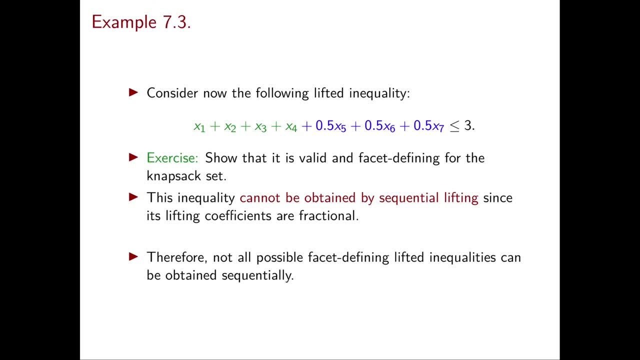 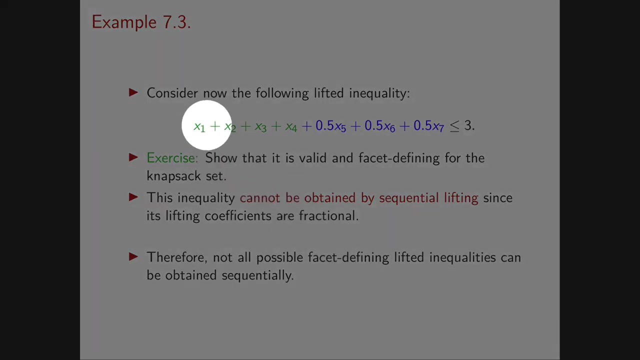 lifted, you may obtain different lifted inequalities. now, an interesting question that you could ask at this point is: can you obtain any possible lifted inequality with the sequential lifting? and the answer is unfortunately no. so this is just an example to convince you of this fact. look at this inequality: it's x1 plus x2 plus x3 plus x4. 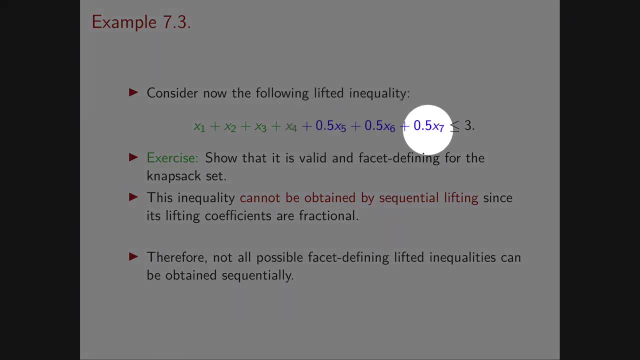 plus one half x5 plus one half x6 plus one half x7, less than or equal to three. by definition, this is again a lifting of our original minimal cover inequality and you can check that if it is not only valid for the knapsack set but it's also facet defining, however, this inequality. 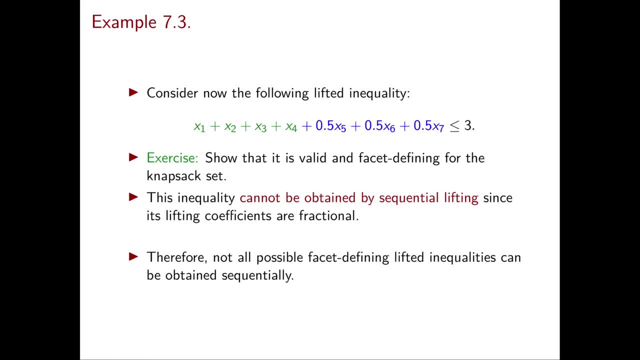 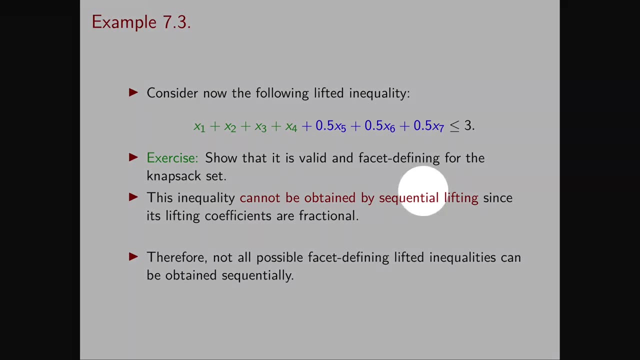 cannot be obtained by sequential lifting. well, there are several ways to see that. you can either try every possible sequence, which essentially we've done, but there's also one very quick way to note that, in fact, by construction of sequential lifting, all the coefficients that you obtain in the lifting process are integer, so you will never be able to obtain four or